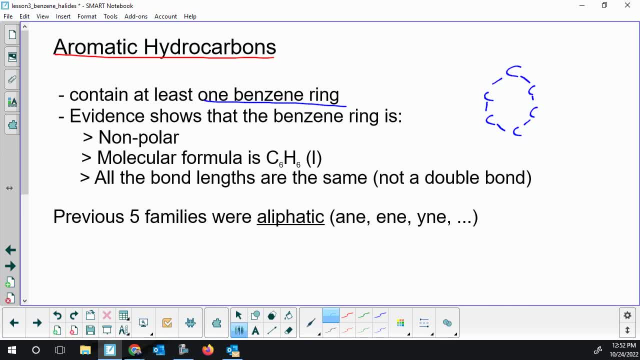 even draw this yet. but it's some six carbon ring. Now, this ring is nonpolar, so there's no positive and negative end. Okay, Okay, Okay, Okay, Okay, Okay. We've got six carbons which I drew and we've got to put six H's in it, That L just. 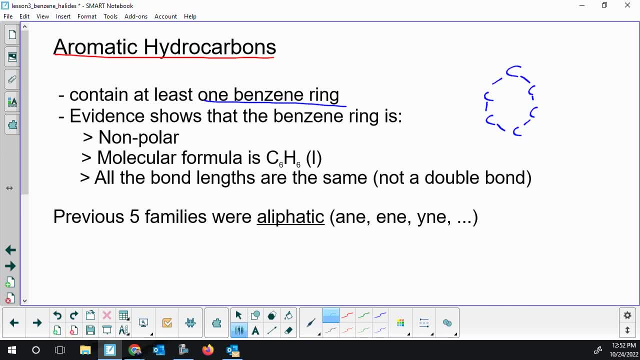 means it's a liquid at standard conditions And all the bond lengths are the same. Evidence shows there's no double bond. There's only something else. I'm not going to say a single, but there aren't any double bonds. Now, everything we did earlier is referred to as aliphatic, So this word didn't come. 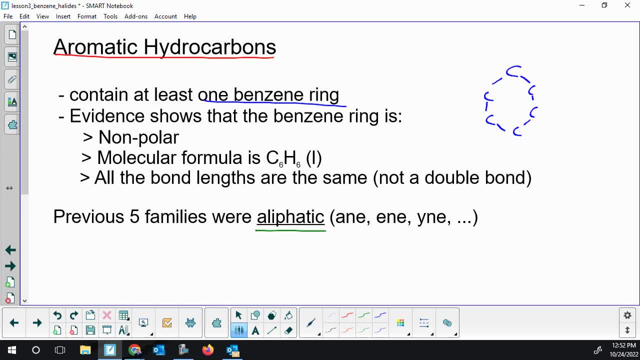 into question. This is a very popular word. It's a very popular word If you have a hydrocarbon or a non-hydrocarbon, or a specific type of hydrocarbon or a specific type of hydrocarbon and you don't have one of these special rings. so that would be our ain family, our een. 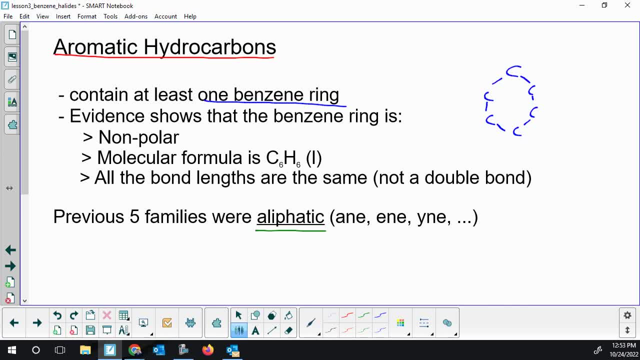 family, our ein family, and I didn't type out the cycloanes and the cycloenes, All of those you need to identify as aliphatic. If it has a benzene ring, you identify it as aromatic. So what's this ring look like? I'm going to put together a little bit of a picture of 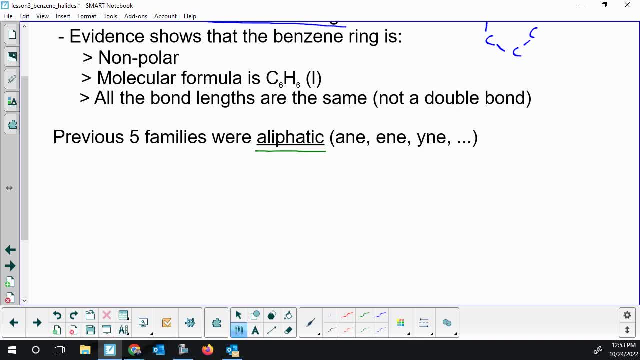 this evidence. so I'm going to start with that. six membered rings, and you would want to draw this in: in order to be a ring, they need to be all connected. that's kind of where I left off from my diagram above. there are six ages. there's. 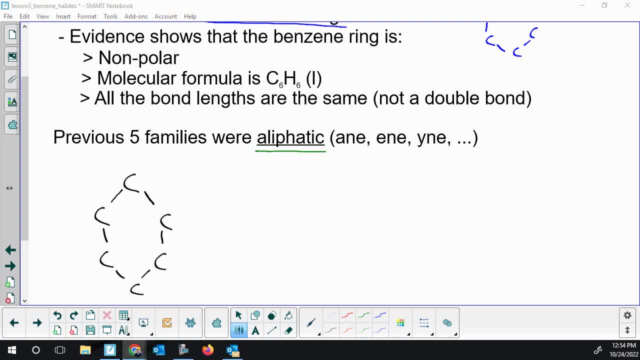 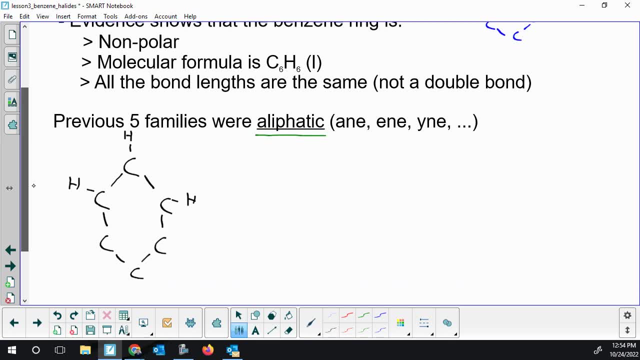 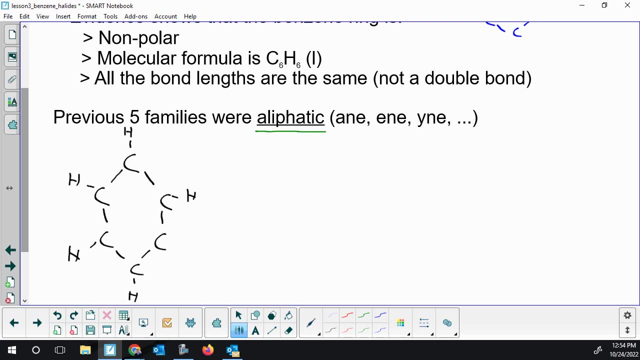 six ages, there's six carbons. you might guess, and you'd be correct, that every carbon has an H. that's what we see when we study the structure. put that in and put that in so that has the right molecular formula. that structure doesn't have any polarity in it. but it's not quite right if you think back to. 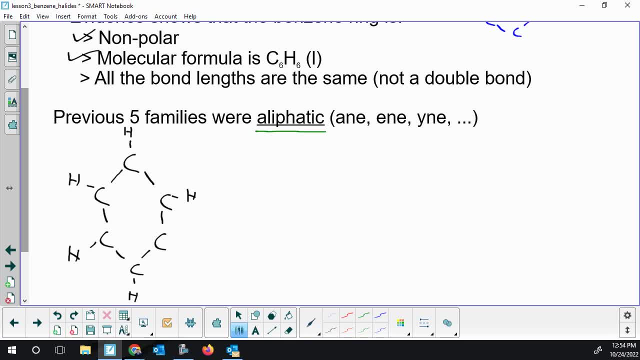 chem 20. how many bonds does a carbon need to have? and then we reviewed it. yeah, it's, for carbon is in group 4a. there's four single electrons and I do not have four bonds. I'm going to get this to work by using your chem 20 skills. if you put a double. 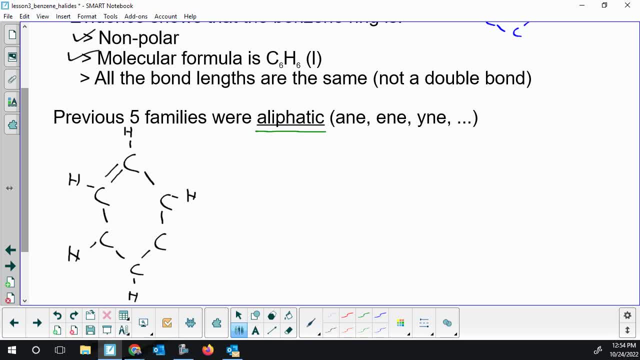 bond in, you get the two carbons around that double bond to have four bonds. so it follows everything you've learned about in chemistry 20. and then, if I double bond the bottom left, I fix those two carbons and then in the middle on the right, if I double bond, there all the chem 20 skills nicely come together. we 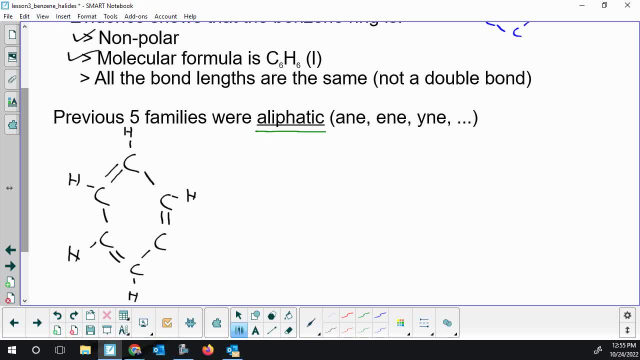 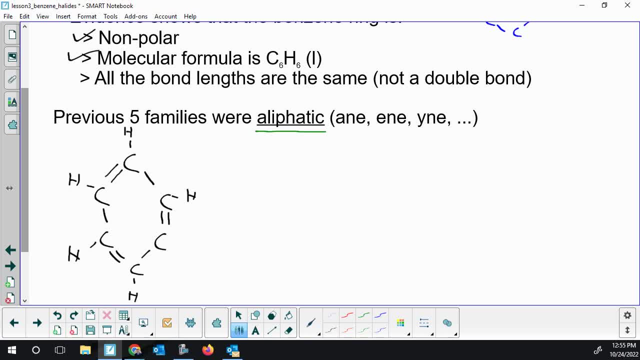 that's kind of right. but where I put those double bonds I started on the top left. I could have started on the top right. I just made a choice to go top left. let's put the double bonds in the other place and trust the other drawing. So I'm going to redraw. There's my six carbons. I'm going to connect. 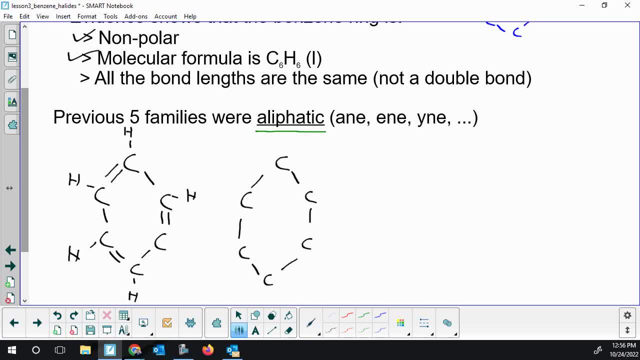 them all in a ring. I'm going to put my six H's in, And now, instead of top left, I'm going to go top right with the double. Pretty much the same, but it's not exactly the same. I flip-flopped. 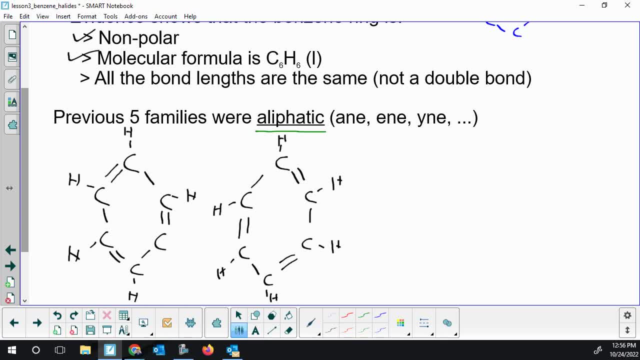 all the doubles and singles. Both of these follow our Chem 20 bonding rules. We have two different ways of drawing the same structure. Now, the true answer to what benzene really looks like is the average of the two, And this is the average of the two. 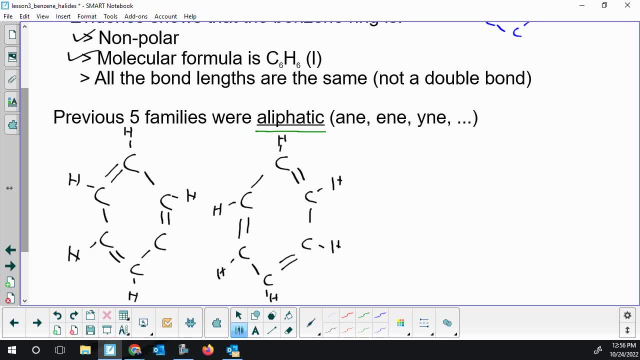 This is something you haven't studied before. It's called resonance structures. It's when you average two drawings out. You're not going to get tested on resonance structures, but a typical nomenclature or way of displaying resonance structures is to add two or three drawings together and put square. 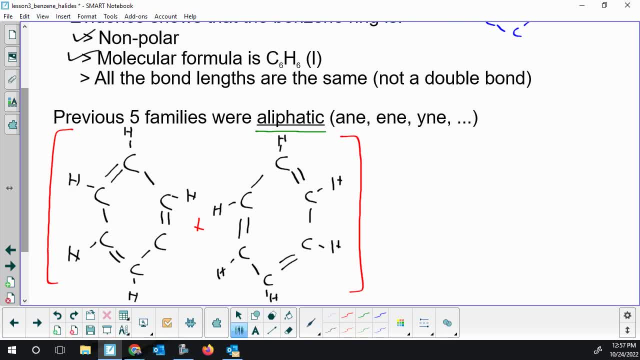 brackets, And we're going to talk about what you would get if you average these two, because that is the truth. That is the answer you need for this course. So I'm going to put a little labeling in. I'm going to put a little labeling in. I'm going to put a little labeling in. 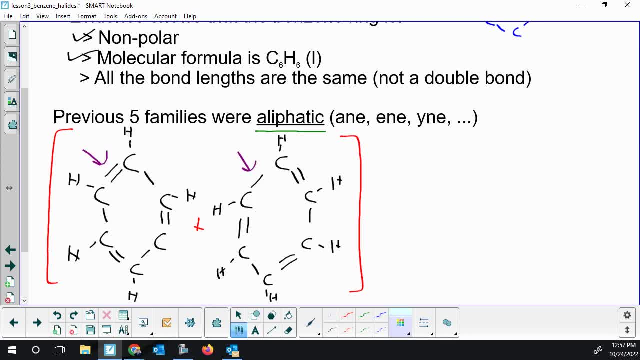 I'm going to average out the top left And the average again is the truth. How many bonds are there on the top left in real life? So any average is: add up all the things you want to average and divide by how many pieces. If you've got 80 on one test and 60 on another, you'd add them two up. 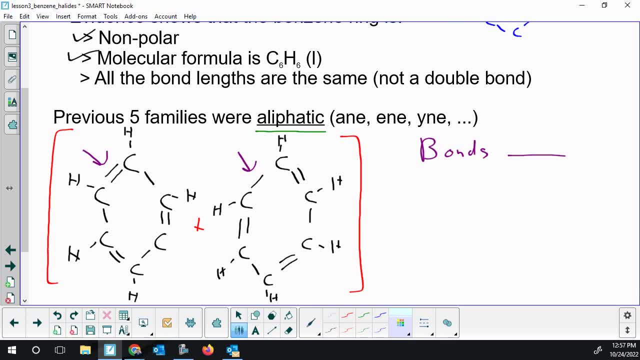 and divide by two. I'm going to do the same thing to get the true picture of the bonds at that purple arrow. So how many total bonds are there where those purple arrows are pointing? Two and one, A double and a single. So there are a total of three bonds between the two drawings that we're going to average And 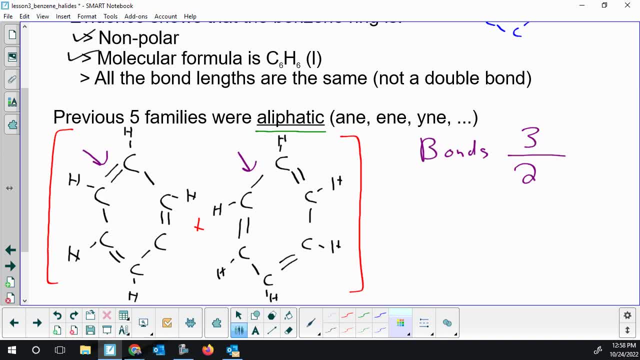 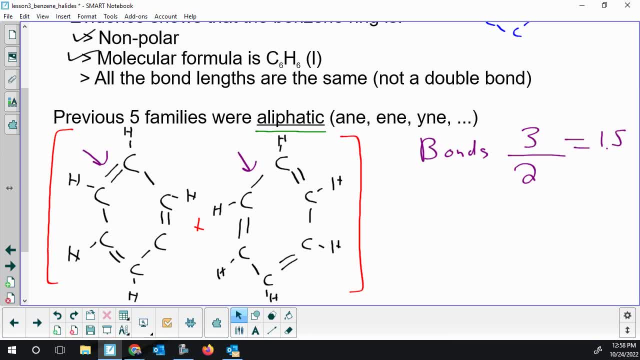 of a bond and a half. I could look at the top right and I get the exact same math. There's three bonds, where those green arrows are pointing, divided by two structures. You get a bond and a half. So all the bond are the same. There's no double bond. There's actually a bond and a half on average. There's a single. 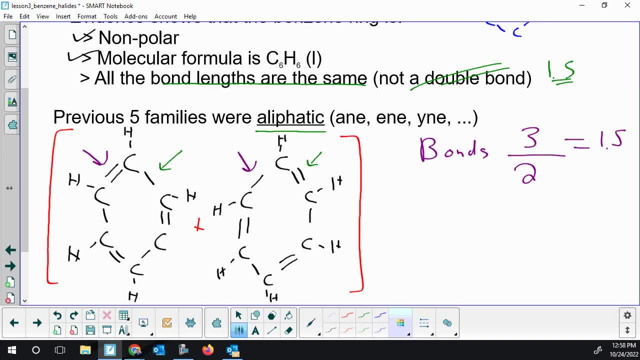 bond and then an extra electron, kind of going around the structure at each of those bonds. How many electrons are in a bond from Chem 20? I write a dash and that means two electrons. So what would a bond and a half be? That'd be three electrons. So I'm not talking about half an electron, I'm talking about half a bond. 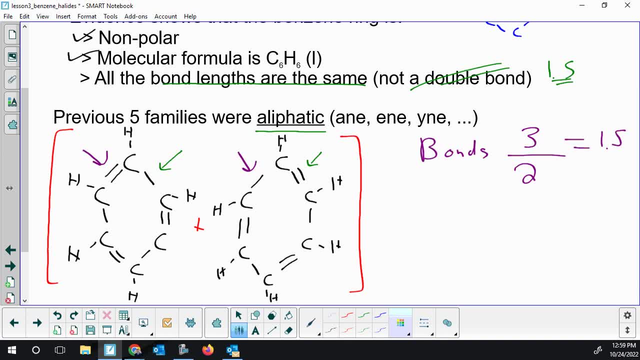 which would be a bond and a half is three Or half a bond would be one electron. So you have these kind of delocalized electrons going around the ring. They average out to one and a half bonds. We're later going to study chemistry that eanes do with full double bonds. 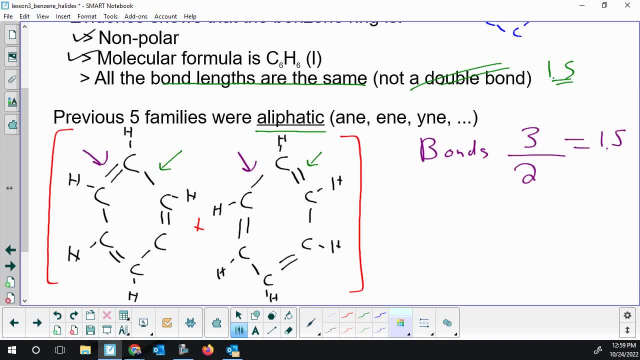 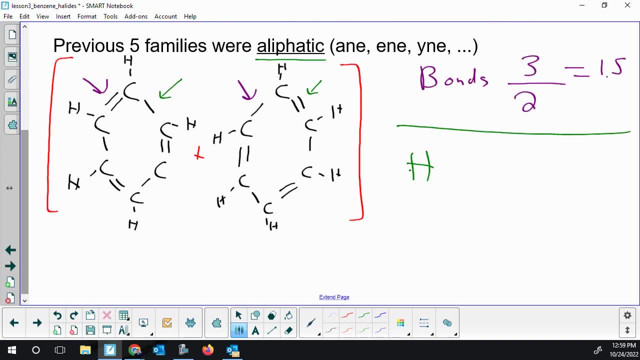 These compounds do not do chemistry that double bonds do, because they don't have any typical diploma question about this is: what is the number of double bonds in benzene? and there's only one acceptable answer: zero. there are no full double bonds in benzene. one and a half is not a double. now chemists have no drawing for. 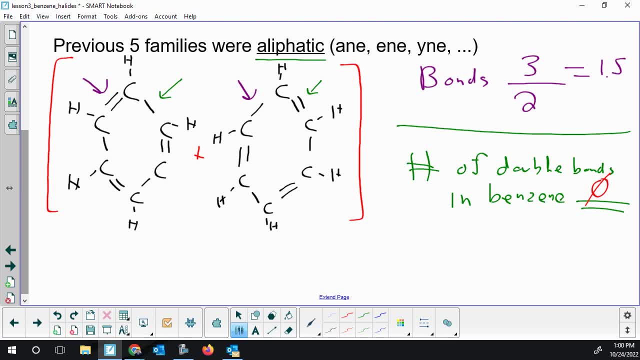 a bond and a half. it doesn't exist. so when we draw aromatic compounds, you could use the drawing I did on the left, you could do the drawing on the right, but both of them are incomplete. if you do the either of the drawings, you think there's three triples, but there are zero triples when you do the average of both. 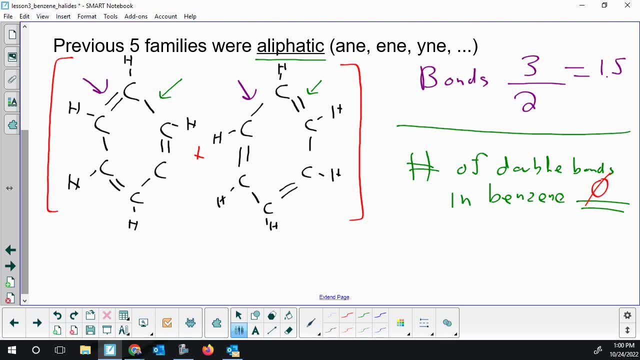 structures. I'm spending a lot of time on this because it's one of the outcomes of this course. you will be asked about the structure of benzene on an exam. it's not a secret, it's just one of those things you must know in chem 20. now there's a 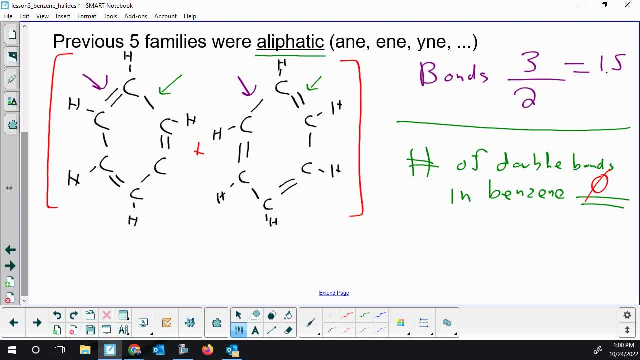 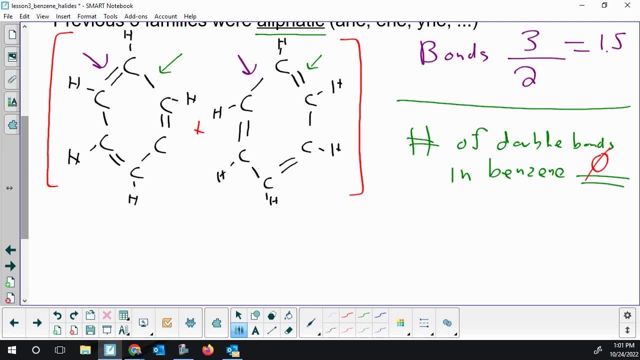 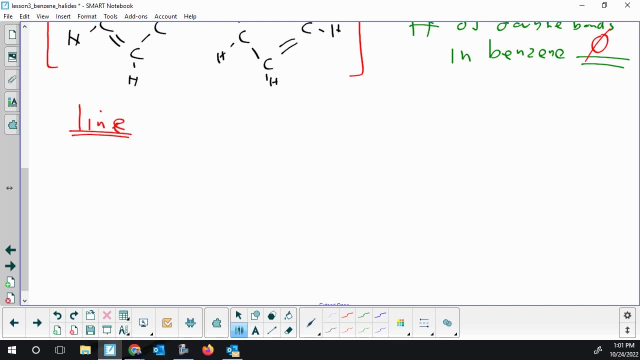 few ways to draw this structure. you've seen two structural diagrams, the left, the right. those are both acceptable. okay, they're kind of annoying to draw, they're time-consuming. so you see, the line structure used a lot and there's two versions of the line structure now. 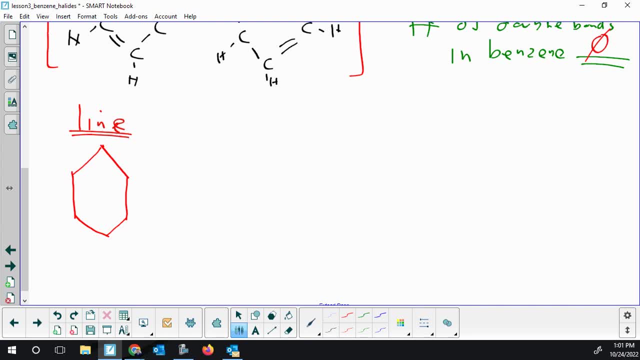 I'm not quite done. this is the heart of one of the versions, if I don't write it anymore. that's cyclohexane, six carbons. there's six line segments meeting six in a ring. But to say that this is benzene, you will see a circle put in. 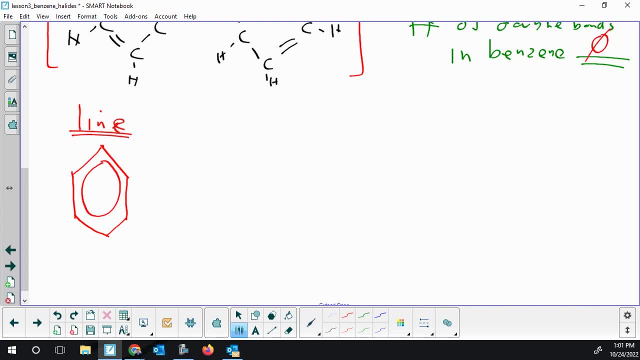 We got that half a bond all the way around and the circle kind of represents that delocalizer, that spreading out of that extra electron going around the ring. So that's one-line version. You might also see it with the doubles, which again is a bit of a lie. 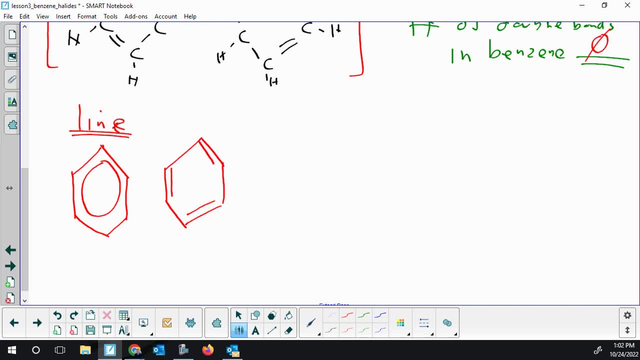 Double, double, double. There are zero double bonds, even though I drew in three double-line segments. We're not trying to trick you. This is what you're going to see in any university textbook is you might see that double, single, double, single, double, single. 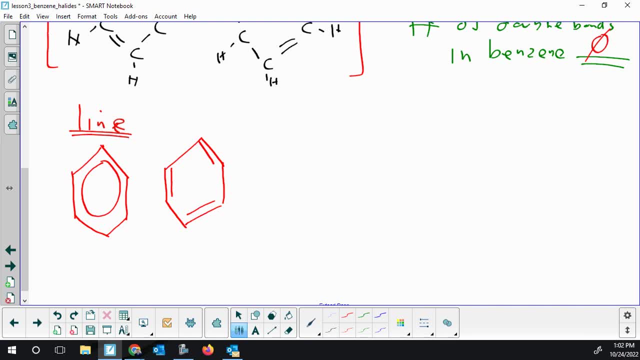 and you need to understand. there's none there, So everything there is benzene. We've got the structurals, We've got some lines. You're not going to see a condensed structured structure of benzene, at least not benzene by itself. 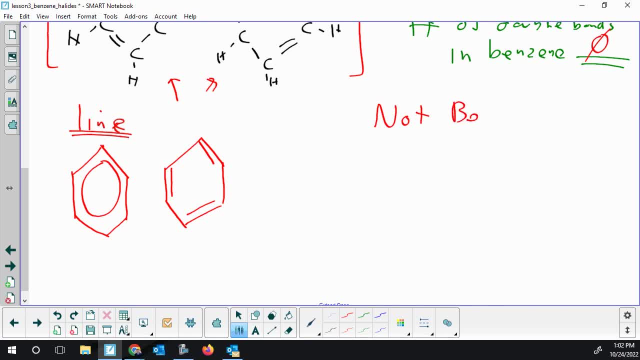 I'm just going to end this slide for some things that are not benzene that I, or an exam or diploma might try to trick you with. You might see that kind of six-membered ring and I might throw in one double bond. 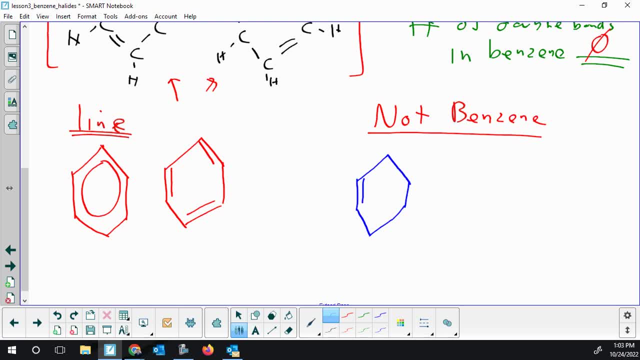 We've seen this already. That's aliphatic, That's a cycloene, One double bond in a ring. You know the pattern. This would be CnH2n-2,, would tell you, would predict the hydrogen count. 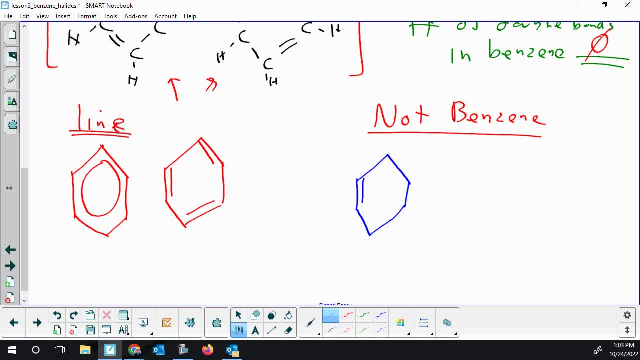 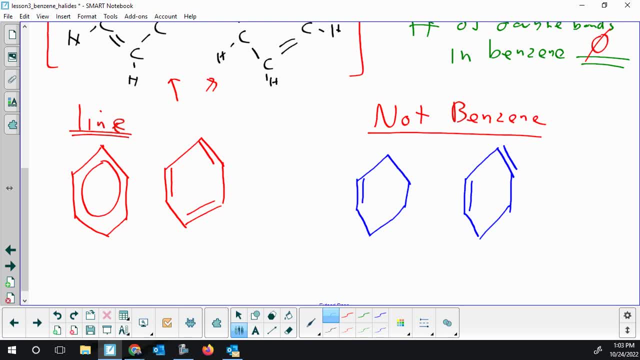 And throw in two double bonds. We never name these. I kind of orally, have hinted towards it. That's a cyclo-diene. That's a cyclo-diene Di meaning two double bonds. That is not benzene. You have to have a third one. 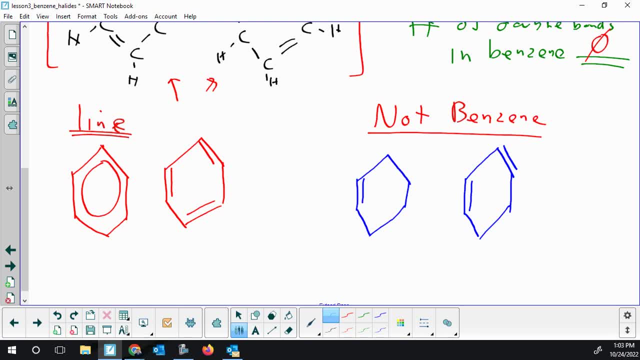 in the right place and get one of the in the right place and get the red structure. So, on purpose, I spent a fair bit of time talking about the structure of benzene, Because you're going to get assessed on it And then we're going to go back. 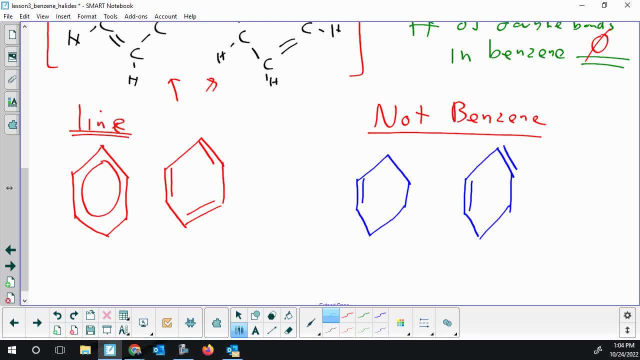 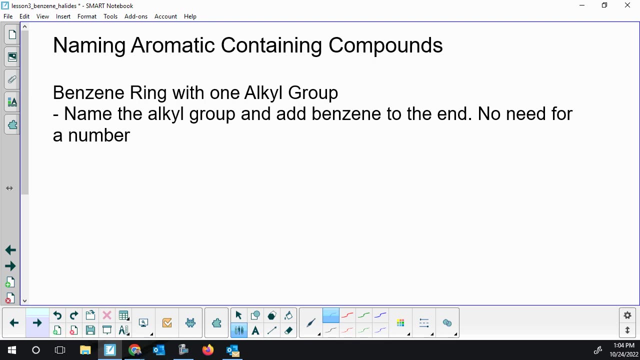 into the heart of what we've been doing. Drawing and naming is what's coming, So we're going to kind of systematically work through simpler to more complex aromatic hydrocarbon naming. So my theme for the next several slides is naming aromatic containing compounds or aromatic compounds. 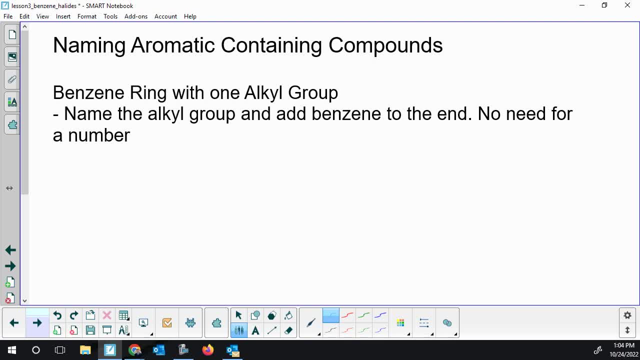 compounds or aromatic compounds. I'm going to start with a benzene ring with one alkyl group. This is going to be very similar to how we named one alkyl group in any of the other rings. We're going to name that alkyl group. 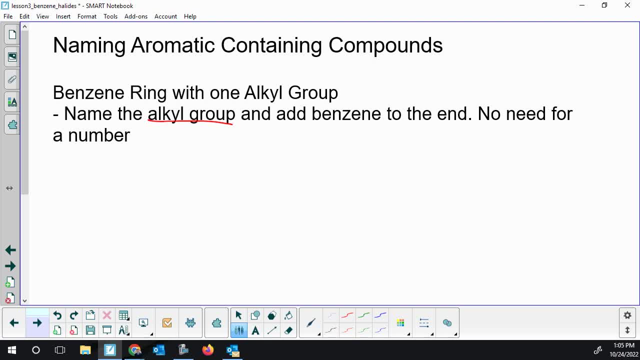 methyl, ethyl, propyl butyl, And we're going to add benzene to the end. No worry about stem or parent or endings, We're just going to stick benzene to represent that aromatic ring that we drew, The six carbon ring. 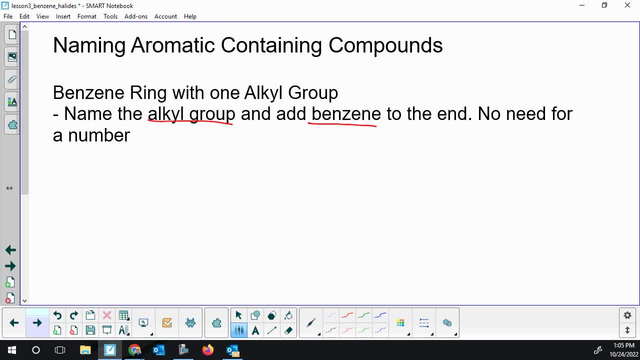 Rings don't have beginnings or ends, So our alkyl group is going to be in the one position by definition and we're not going to put the number. So I'm going to do a bit of a mixed drawing. I'm going to do the line structure. 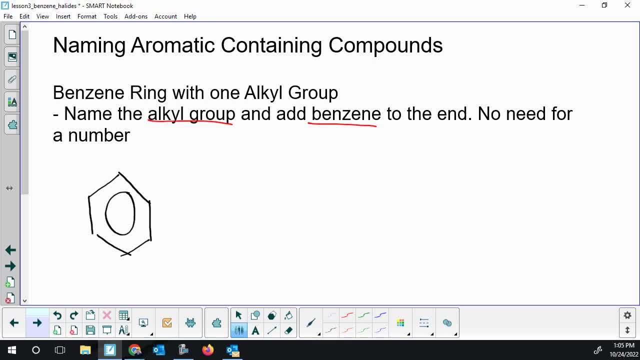 for benzene because it's easy to write, It's clear for students. But then I'm going to do a structural diagram of my branch And I'm going to do a two carbon long branch. Every one of those carbons needs to have. 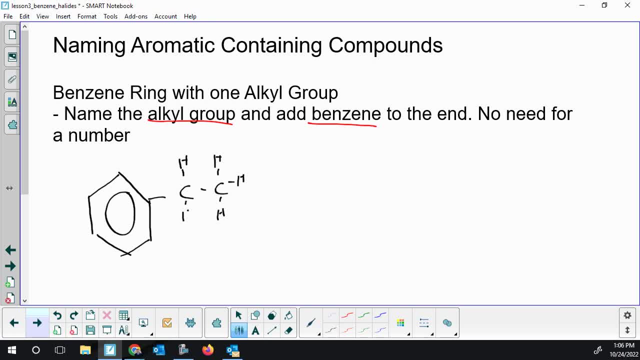 four bonds, And our goal is to name this Now, the heart of this drawing. you have to recognize this ring As not being a cycloane or ene, but being benzene. One of those six membered rings, Now one. 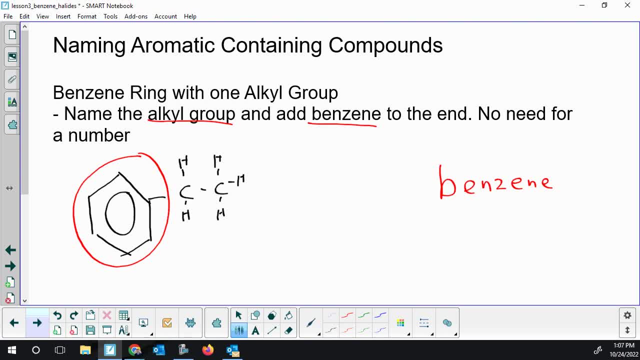 of the H's was removed and that's where the anethyl group was added in. Then we deal with our branch. I always box up my branches. That is a two carbon long branch. So that is ethyl. We're going to put it in the one position. 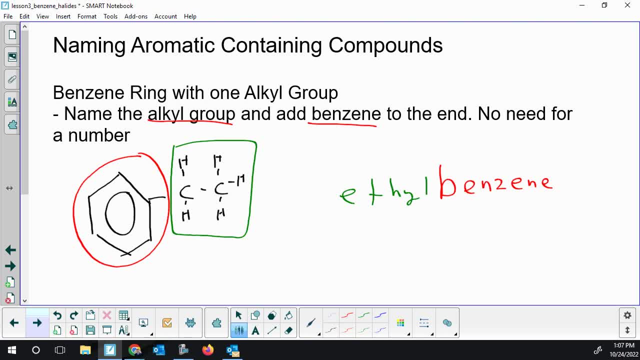 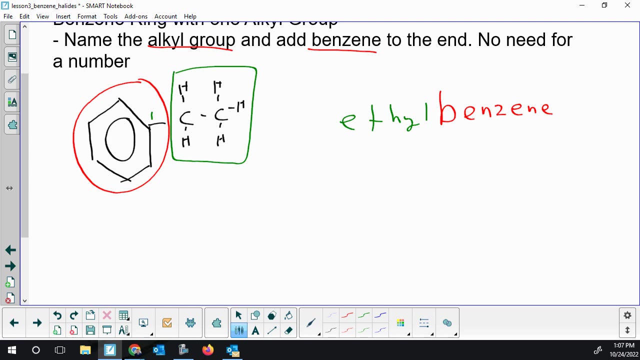 But we're not going to put that number in. And that's it for the name when there's one. So that's it. We're going to put it in the one branch. I'll do the full line structure. So I already had done the. 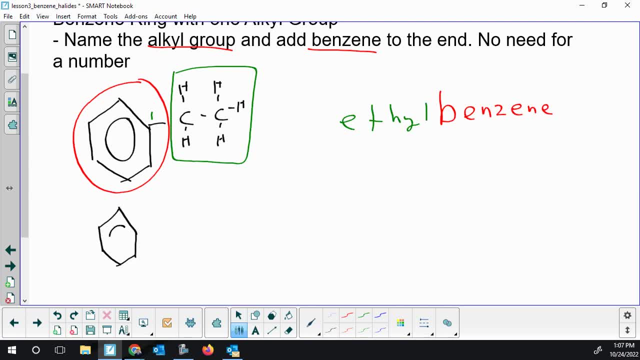 line structure for the benzene ring And then I have to show two carbons coming off of it. Now, when I do branches off a chain before I would drop my pen and zig and zag, I drop it and say one, two, three. 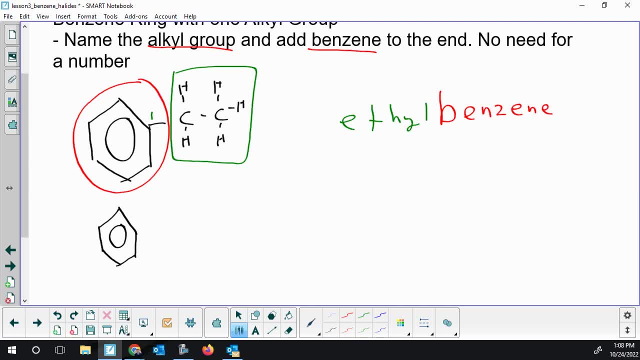 four, When you do a branch, when you drop your pen, I'm going to say zero, because I'm already on a carbon. That's not a new carbon. Zero, one, two lift And that will get me two or an ethyl. 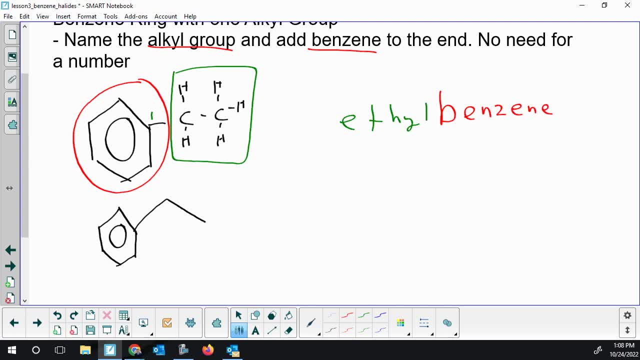 So I dropped on top of an old carbon and said: zero, one, two done. I'm going to erase this, but my strategy for students with line drawings is to put circles everywhere lines meet, And that's how you could get out the carbon. 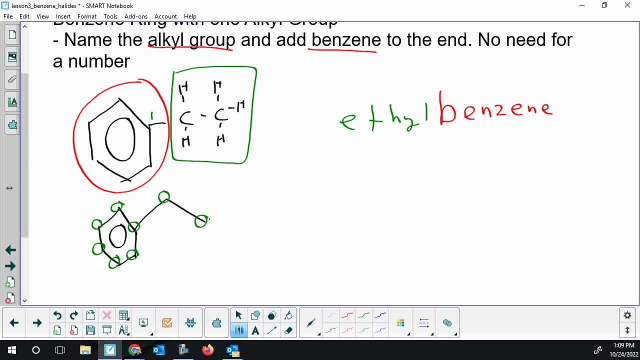 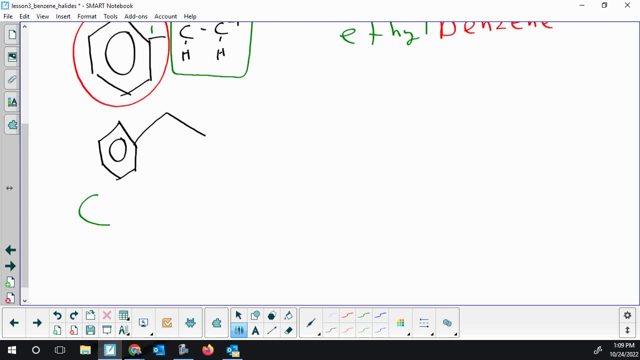 count. There's six circles on the ring and then there's two green circles off the ring. I'm going to take those out of my diagram. I will do the molecular formula. We don't have any generic pattern here and it's a very common diploma question. 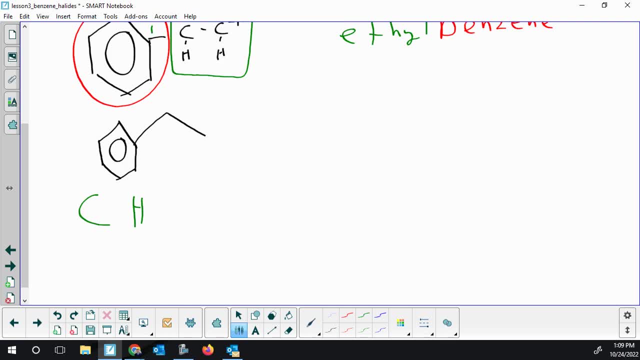 Almost every diploma has what is the molecular formula of something, particularly line structures. Now, how many circles did I have before? I had six in the ring and then two for the ethyl. So six and two, that's eight carbons. Molecular formula is just a count. 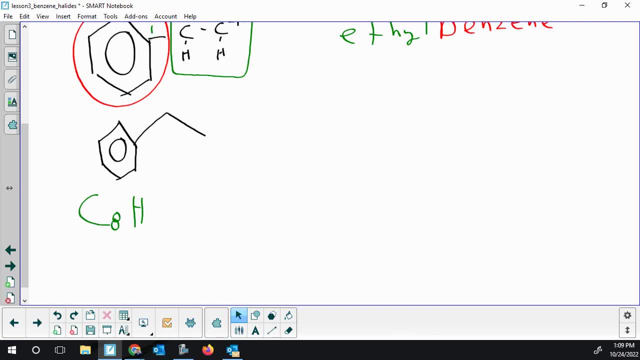 And then we're going to need to correctly identify all the H's. I'm going to put a check mark for every H as a visual to count. So this top would have one hydrogen. There's one here, There's one there, There's one there. 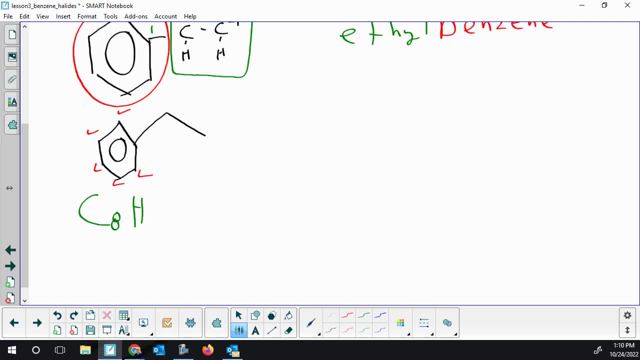 There's one there. I'm going to erase this. There is not one there because we put a branch off. So that would be an error you might make analyzing line structures of benzene. Where a branch came off, there isn't room for another. 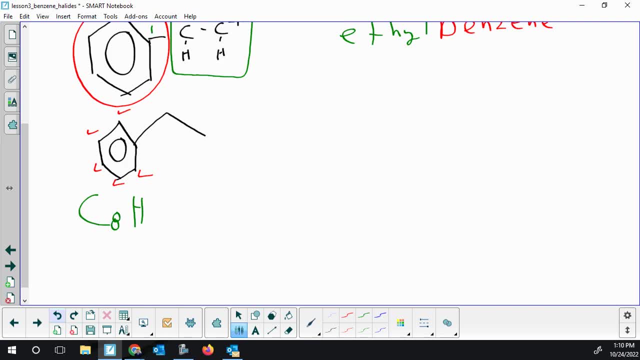 or a fifth bond, because there's a bond and a half on each side of the ring. So that's three, And then the ethyl coming off is the fourth. We have a line segment, The first line segment, meeting in our ethyl, And here 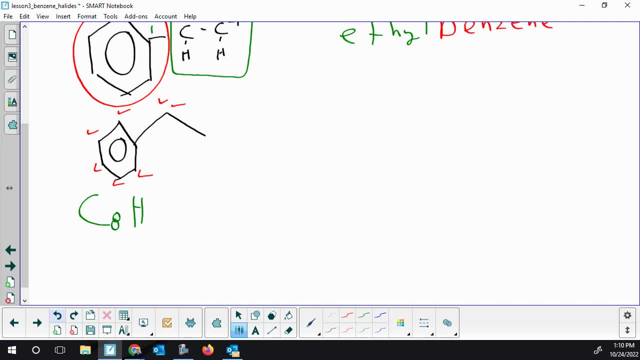 there would be two H's And at the very end there would be three. Now you might need to draw this out structurally if you're not quite seeing it, as I check them off, But that's the correct count. So what am I at? One, two, three, four, five? 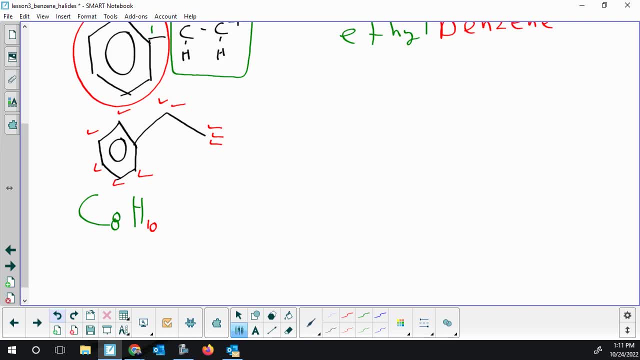 six, seven, eight, nine, ten, Seven H's In ethylbenzene. So that's benzene with one alkyl group. We're going to go benzene to two alkyl groups, but I'm going to keep them the same. 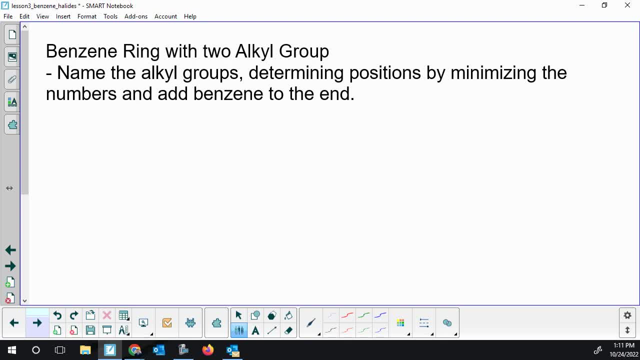 The rules are really going to get repetitive from here on in. We've done this before. If we have two same alkyl groups, we're going to use di and two numbers. We are going to need numbers to tell the reader how far apart are they? Where are? 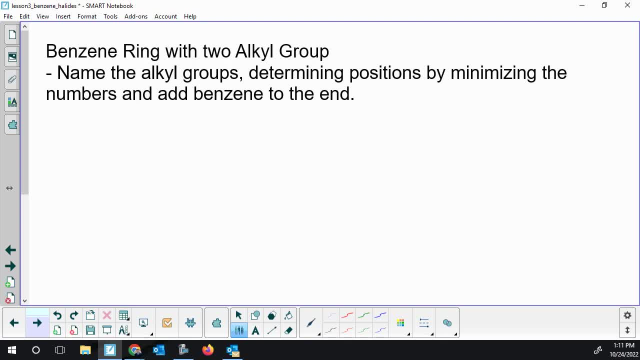 they? Are they neighbors? One? two, Are they as far apart as they can be, Which is one? four: I want to do some line structures That's as close as they can be. You can't have them off the same. 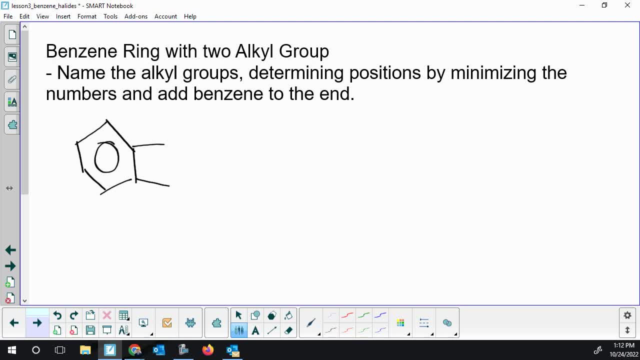 carbon, because there isn't enough bonding capacity within the ring. What you need to remember is that that single line is actually one and a half bonds, And that's one and a half bonds. So the black line coming out of the ring is the fourth and last. 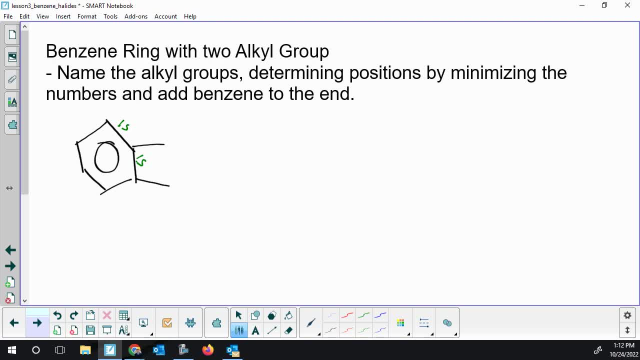 possible bond. If I kind of box up my branches coming off, there's only one end of a line segment in that box, So that's a methyl And that's another methyl. There's only one end of a line segment, So we have two methyls. 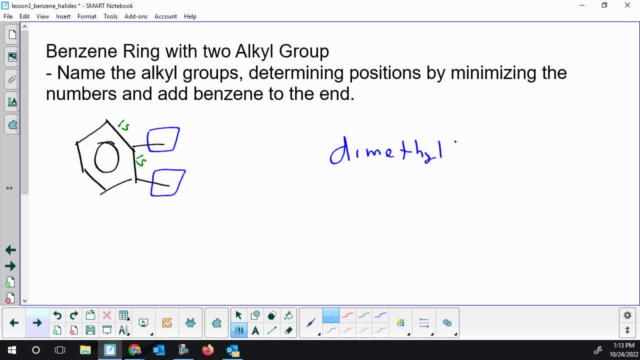 Dimethyl. They're coming off benzene And we are going to need a couple numbers because they don't have to be next to each other. We're going to pick one as our one position and take the shortest root to the other. So if I 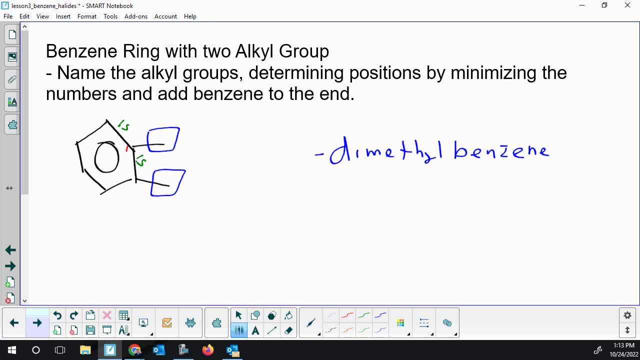 pick that as my one position. the shortest root would be clockwise and that would be my two. So I kind of arbitrarily picked one of them as my one, even if I pick the other one as my one, Now I'd go counterclockwise and that would be my two. 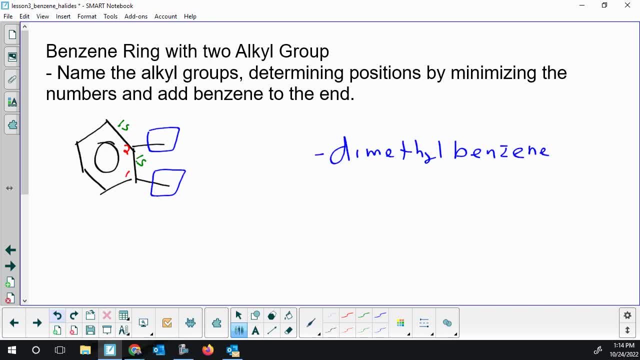 Doesn't matter which one I pick first. If I pick and then minimize the distance, I get one, two, dimethyl benzene, And there are only three options: One, two is when they're neighbors, If there's one carbon with nothing in between the two branches. 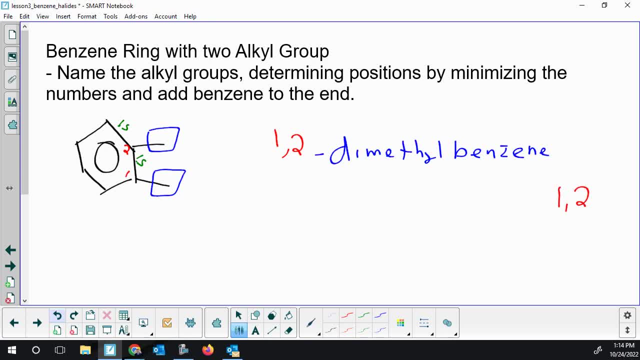 it's a one three. And if one is at one side and one is as far away on the other side, it's a one four. That's the only three number combination. So that's a one three. That's the only three number combinations you're going to see. 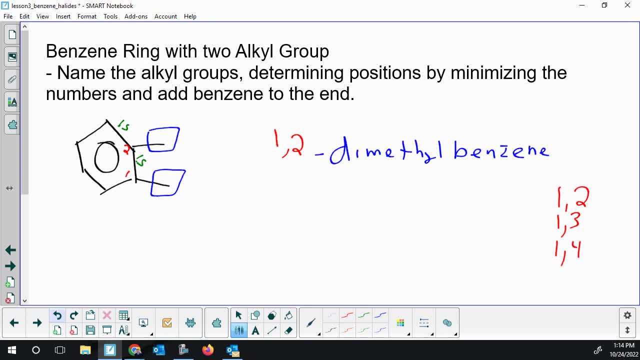 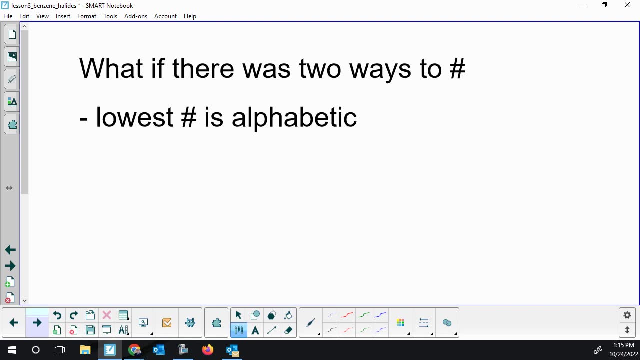 with di something: benzene, dimethyl, diethyl dipropyl. So we're well through two alkyl groups that are the same. what if the two alkyl groups were different? If they're different, we pick as the one and the one we pick. 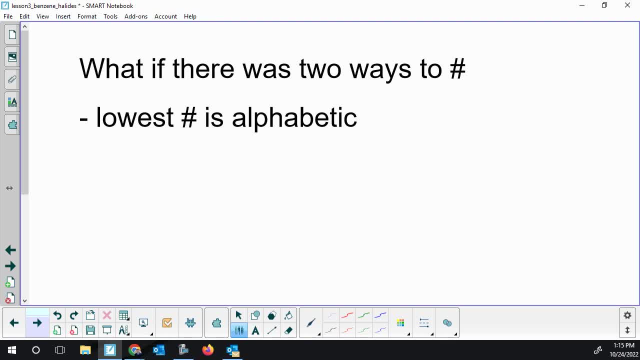 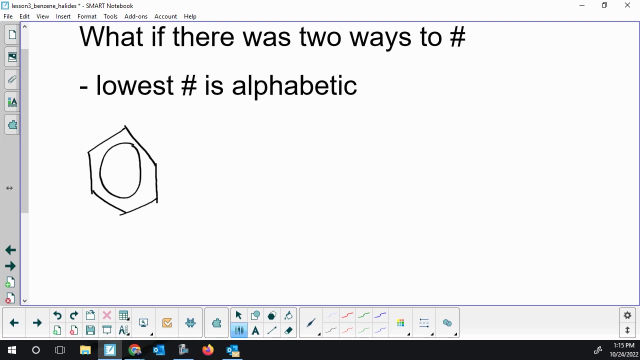 as the two is going to matter, And how are we going to deal with deciding which way to pick if they're different? Well, we're going to go alphabetic. I'm getting pretty used to this line. structure of benzene. I'm going to put a methyl. 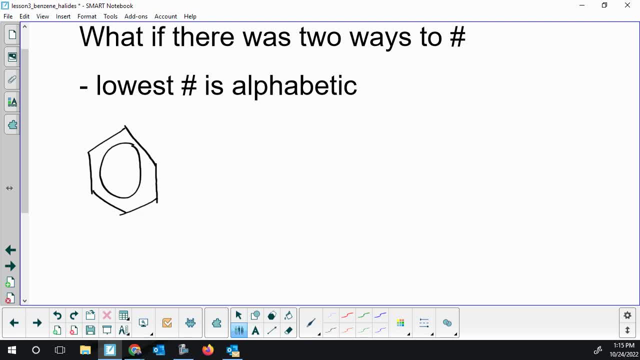 on. I'm going to put a methyl on And hopefully we're going to all do it together. I'm going to drop my pen on an intersection but say zero, because there's already a carbon there. One, lift my pen. I've added in a. 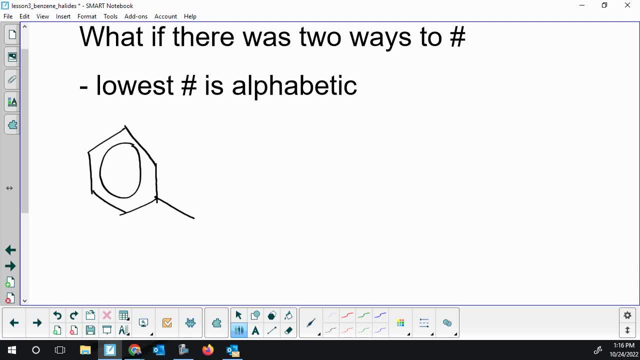 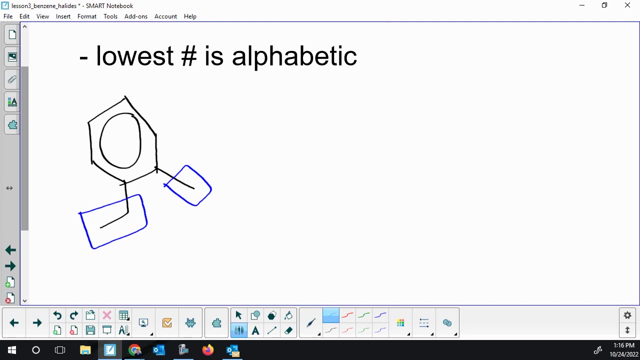 methyl. Now I'm going to put in an ethyl at the bottom, Drop my pen and go zero. one, two lift. So I have two different types of alkyl groups. I've got my one long and my two long. You don't have to add this into your notes. 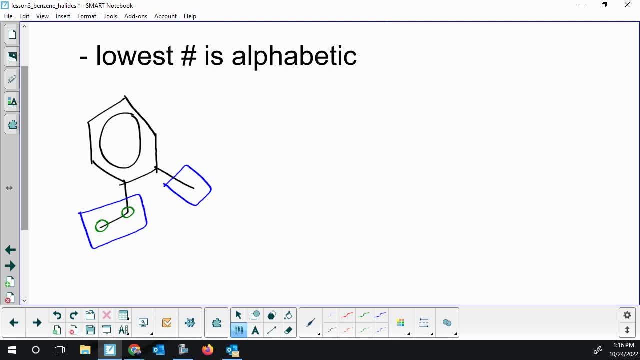 but if you have trouble with the count, put a circle at the end of every line segment. All the other line segments are part of the ring. So those six I added in at the end are what give us benzene. I've got to decide which. 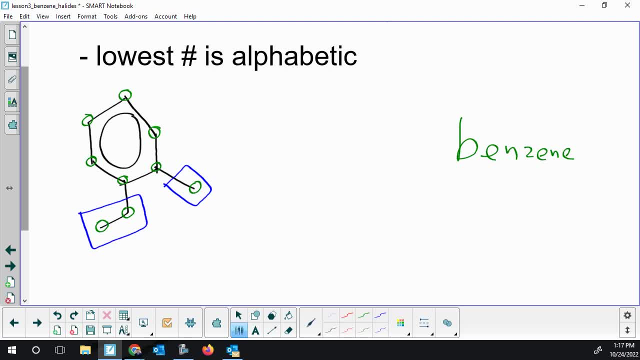 one is going to go in the one position. I'm going to go alphabetic. So I have a methyl which starts with an M and I have a ethyl which starts with an E, So I'm going to put the ethyl in the. 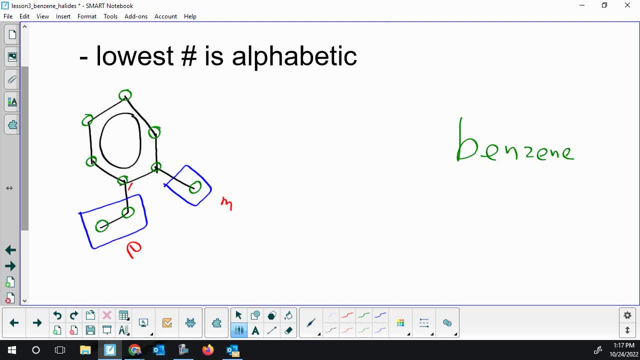 one position and then minimize the numbers to the other. If you had three things, you wouldn't put them all in alphabetical order for their numbering. You'd do the first alphabetic and then set your numbers from there. There are two systems for doing this. I'm teaching. 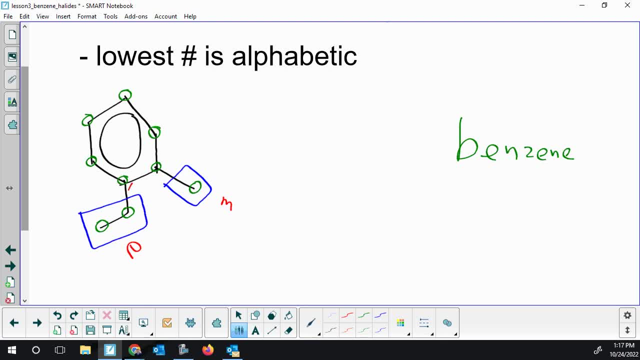 you just one. If you read about the other system and you answer a quiz question with the other system, I will mark that correct. also, Diploma questions won't have ones that there's two different answers depending on the system. So that's the one I'm going to go. 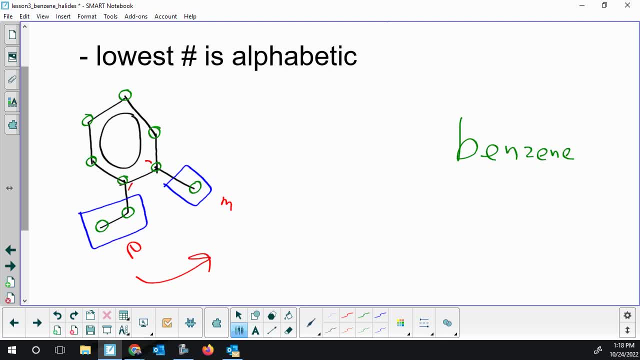 counterclockwise to get to my methyl and that's going to be in the two position. So I have a one ethyl and two methyl benzene And this would be an aromatic hydrocarbon. It is not aliphatic because it has 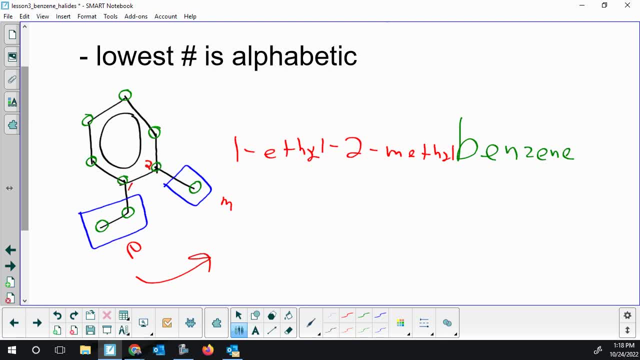 one of these special rings, Not quite lord of the rings type rings, but it is special in terms of organic chemistry. So we're almost done aromatic compounds. We have one thing left. It's kind of annoying. It's a different type of pattern. 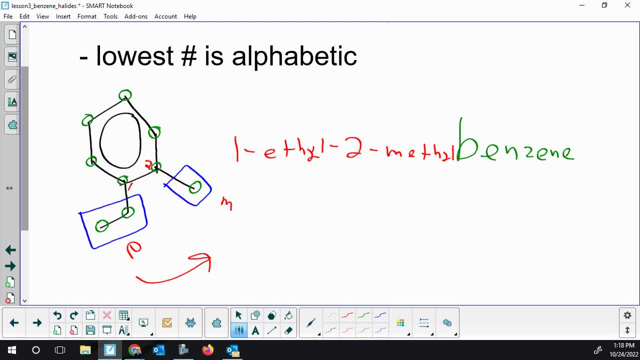 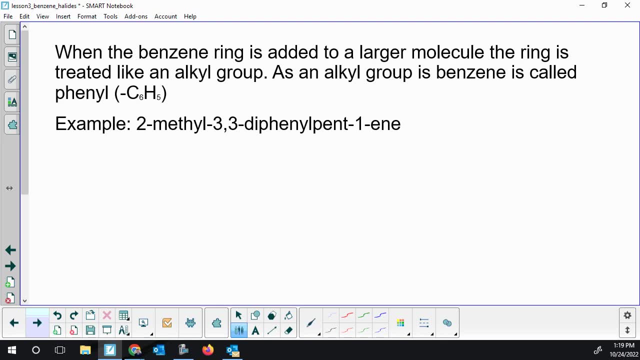 that you have to recognize and name it a little bit differently. You can have a benzene ring. that is itself the branch- And you'll see that in a second when I draw this crazy long name- When benzene is added to a long chain of 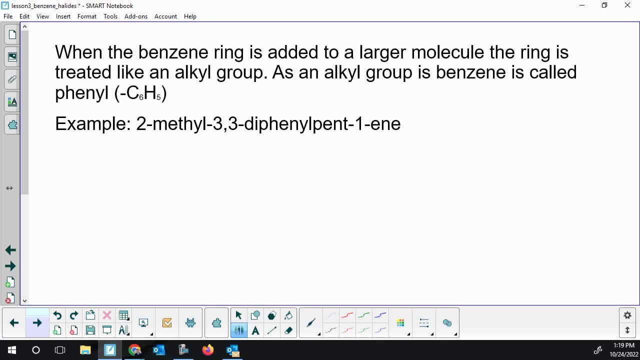 carbons. we treat it as an alkyl group. And when we treat it as an alkyl group, we're going to use a different name for it, Which is kind of a bit annoying, but we're going to call it phenol when it. 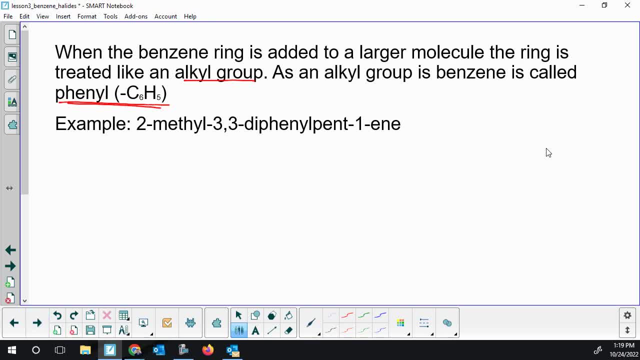 itself is coming off a chain. So before I jump into that name, I'm trying to give you a little bit of visual. What do I mean as the benzene being a branch itself? Maybe you have an eight carbon long chain, You don't even. 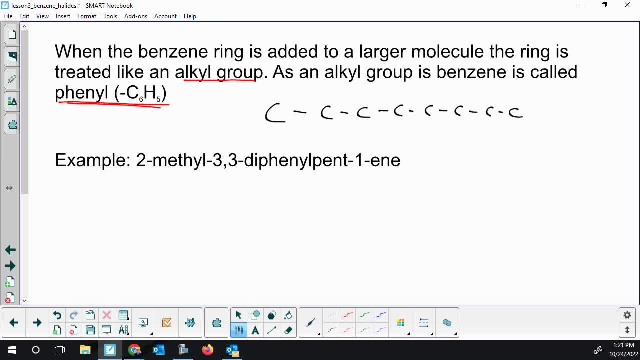 have to put this in your notes- And that chain maybe has a methyl coming off and an ethyl coming off somewhere else, And then further along we've got one of these benzene rings. We're not going to be able to call this benzene and then name the branch. 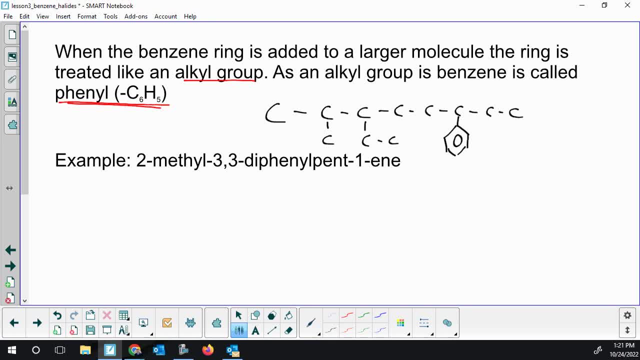 because the branch is going all over the place. When you have one of these rings, that itself is coming off a great, big, long chain, we're going to treat that like a branch And all along we've treated everything coming off of it as a branch. 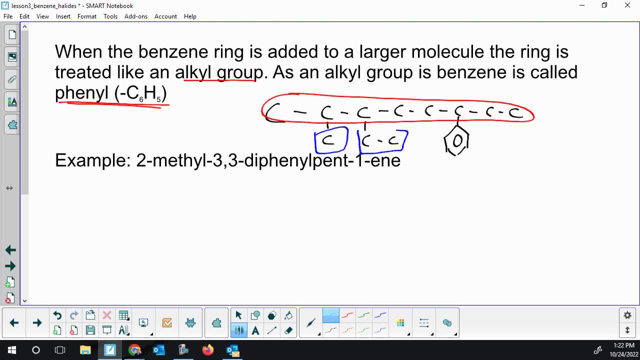 So here, we'd have that methyl, we'd have that ethyl, and then this we're not going to call benzene, we're going to call it phenol. We've got that YL that we're used to seeing with alkyl branches. 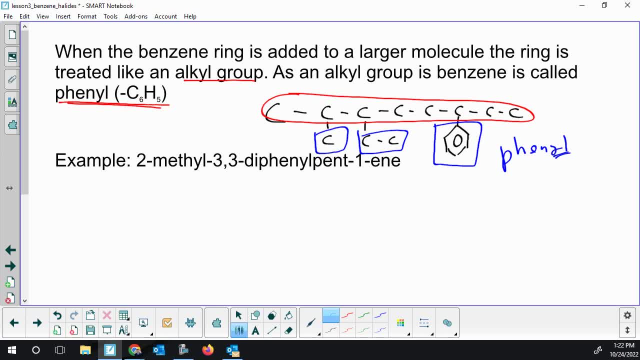 It's not an alkyl branch, but we're going to use the same type of rules and conventions. Our systematic steps are going to be the same. And then I've got an example and I've thrown everything we've learned pretty much into this. 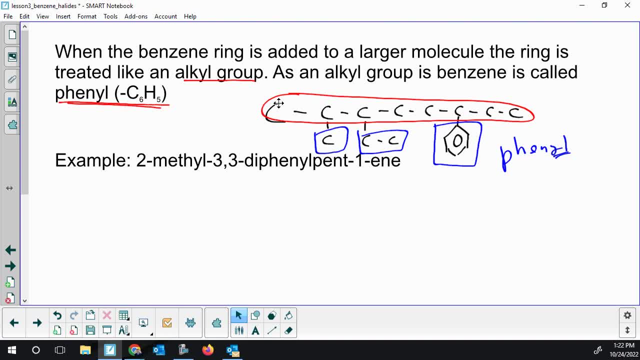 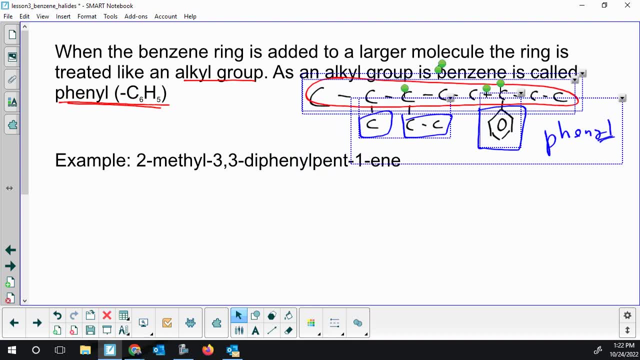 This is as hard as it could get, and I made it really long on purpose, because if you can follow the steps to decode this, its length is irrelevant. You just take it piece by piece. So before I dive into this, I'm going to remind everybody. 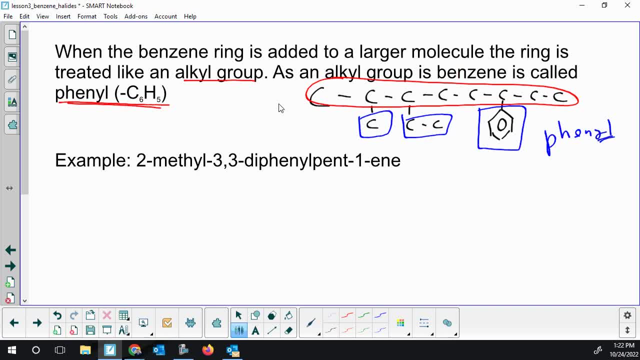 of the order that you deal with. any organic compound, The first thing you deal with is what The stem or the parent. So we've got to start there. Then we jump to the end. So we've got a pent with a double bond. 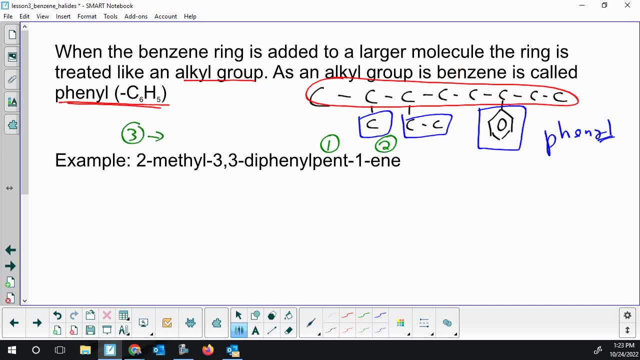 and then we can start working our way through that long mass. but we just do it piece by piece. How do you eat an elephant? One bite at a time. How do you draw organic compounds, One branch at a time And step by step, hopefully. 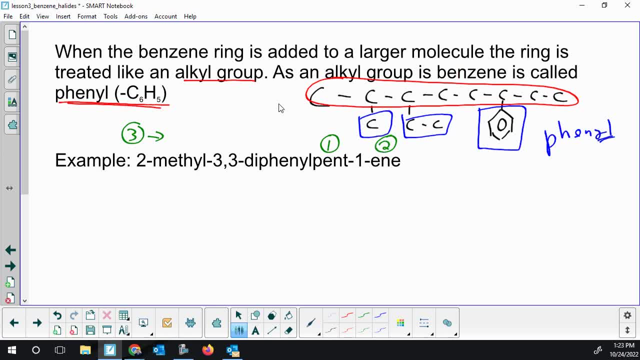 it's not too bad. So step one is pent. One, two, three, four, five. That's step one done. One een First carbon-carbon bond has to be a double bond, So I've got to pick a side. 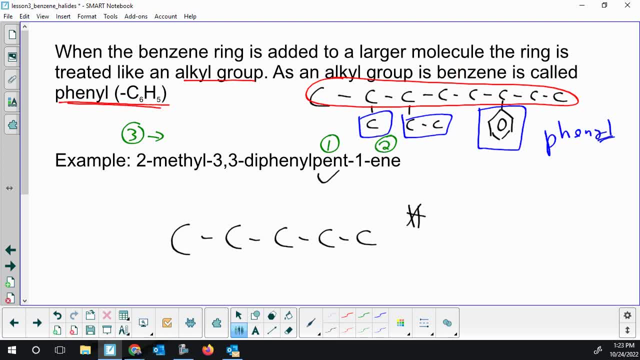 I don't know. I'm standing close to the right, so I'm going to do all of my counting for the whole question from the right. I could have picked the left if I wanted, but I can't flip-flop. I want to put the double bond. 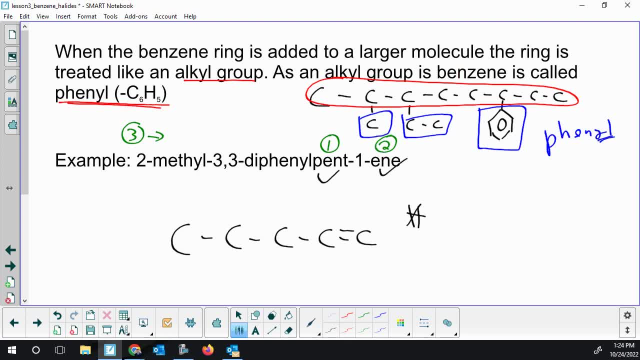 in the one position from the right. So step one and two is done, but I put that star there to cue my brain to keep counting for the right. Now I've got a two-methyl, So my second carbon over has one carbon. 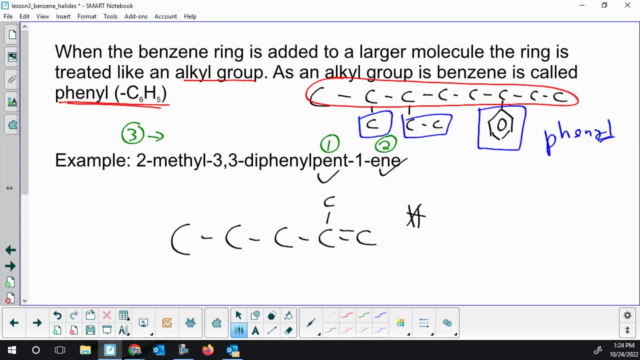 I could have went up or down, It didn't matter. But I'm two carbons over from the right, So that's my two-methyl. Three, three di-phenyl. So now, for the first time, we've seen phenyl in the branching. 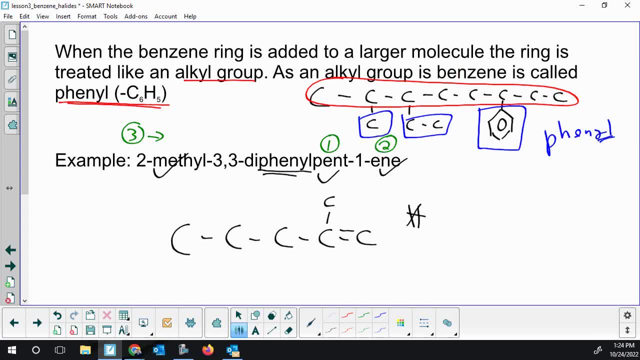 section. So my third carbon over. I need a phenyl. I would never fit in a structural diagram. Your diploma will use lots of lines. That's one of the phenyls. I need a second phenyl And I'm going down. 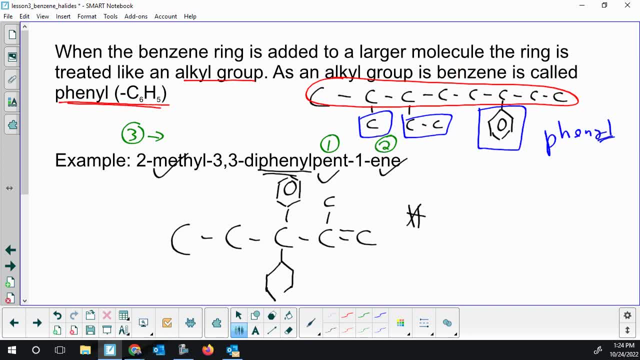 because that's where I have room to put it. They could be both up, both down, one up, one down, It doesn't matter, And I took care of both of my phenyls and then I just used bonding capacity to complete it. 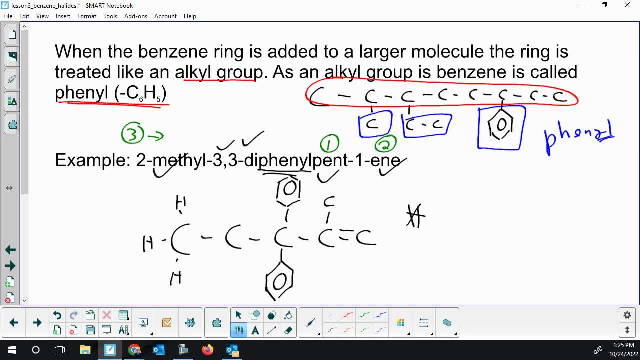 I'm going to repeat my drawing. I'm counting to four for all of my carbons. Where I have the di-phenyl, that middle carbon has four bonds And I'm done So kind of step by step. Now, sadly, 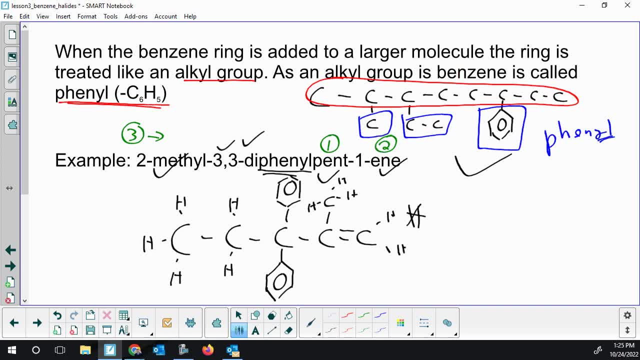 I wouldn't give this to you on a test. I might for homework. I might as an example. Alberta Ed says we're only supposed to assess, giving two parameters or two naming sort of systems. So this one has a benzene ring, It has an alkyl group. 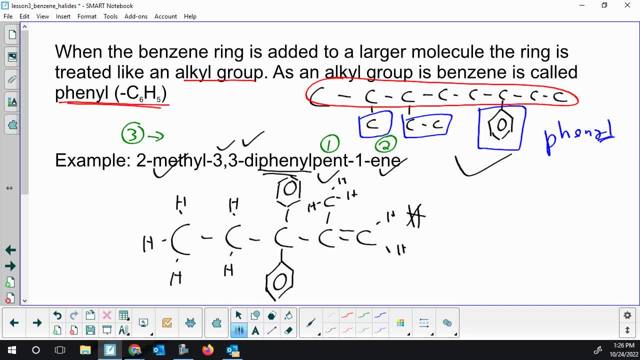 and it has a double bond. So that's three. So that exceeds what we're supposed to do to you. Two: If you were to put in the phenyls and the double bond, that would be fair game on an assessment. So don't worry. 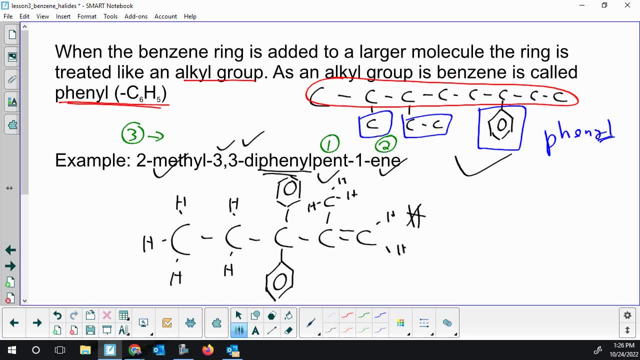 as we build up in complexity, the questions can't have everything put into them. They can have two pieces of what I've taught you. So that's our aromatic grouping. The structure I just put up has two of those rings, As long as it has one. 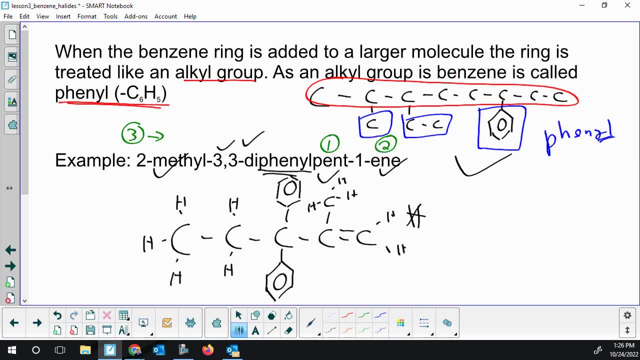 you call it aromatic, You call it aliphatic. Now we can really fly. Aromatic rings are done. I'm going to go into organic halides and this is going to be one slide We're going to add in a halogen. 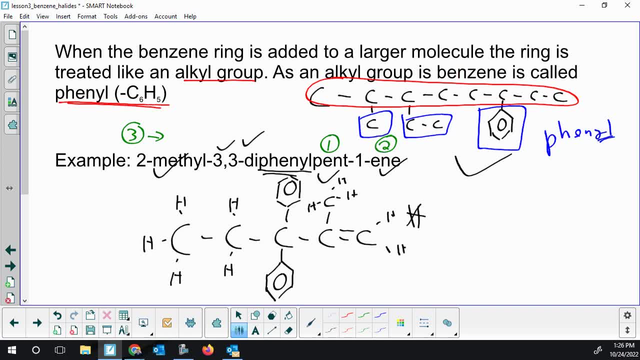 but we know how to number it. We just count from an end. All you need to know is: what name do I use for the halogens? and you can deal with everything. If there's a tie, you're going to go alphabetic. If there's two of them, you're going to put di. 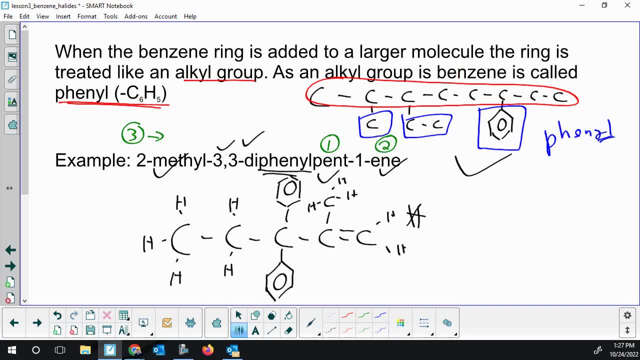 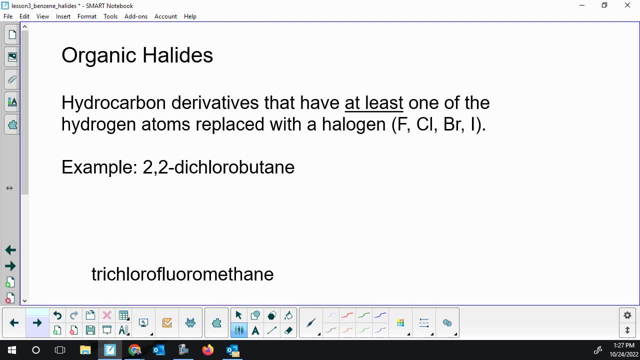 If there's four of them, you're going to put tetra. We're just reusing the rules. Organic halides: Since our very opening slide, I've never talked about a hydrocarbon derivative, because we've never had something other than C and H. 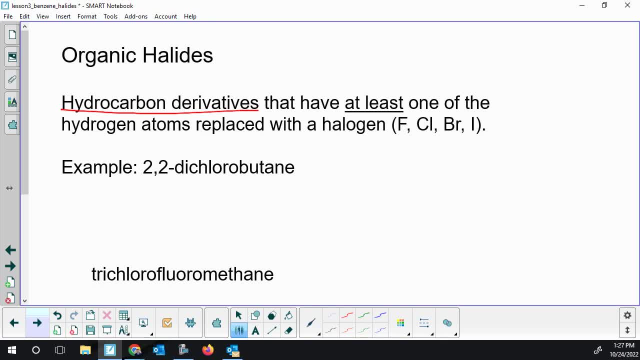 But we will here. Organic halides are a hydrocarbon derivative. They have at least one hydrogen replaced with a halogen, But they could have two or three. All of them could be replaced with halogens. You don't need any hydrogen at all. 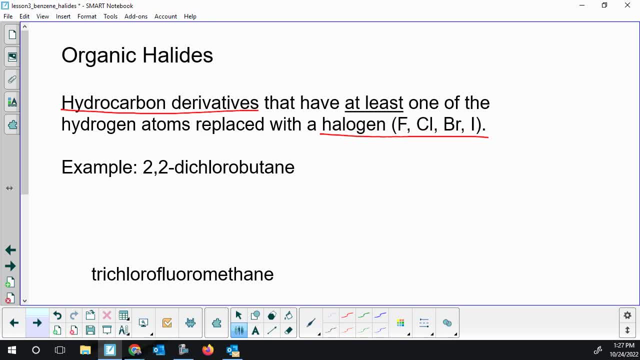 in a hydrocarbon derivative. I'm going to jump right into naming because you don't need rules. You know what those twos mean. You know what butane is, We'll jump right in. I will draw 2,2-dichlorobutane. 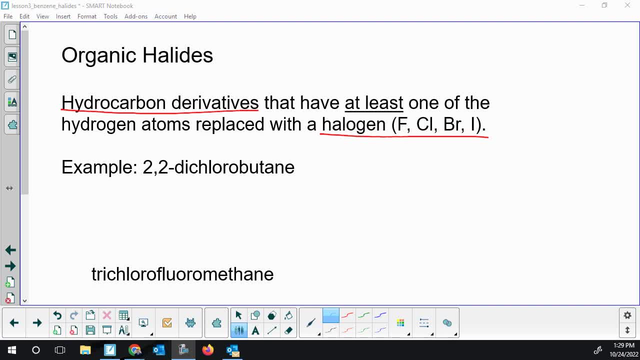 I'm not going to number it, but it's still one, two, three, Stem the ending ane and then we'll go to the front Bute: one, two, three, four, 2,2-dichloro. 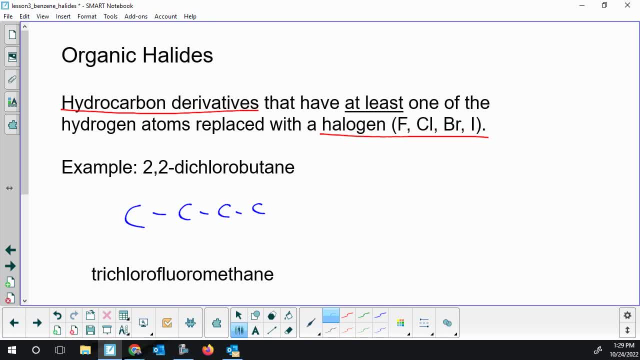 We have two position. two position. we have two. We don't write chlorine. They all end in O. Our halogens are going to be fluoro, chloro bromo and ido, IDO. You might see some nuances if there's two vowels. 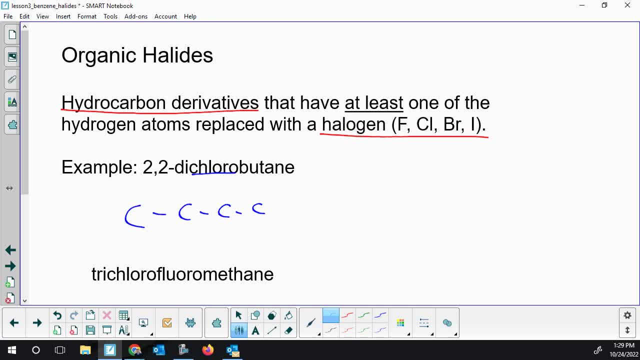 next to each other. You might see them dropped. I have to pick a side. I'll go to the left this time. You could do it from the right. It would be equally correct. There's my second carbon and there's a chlorine. 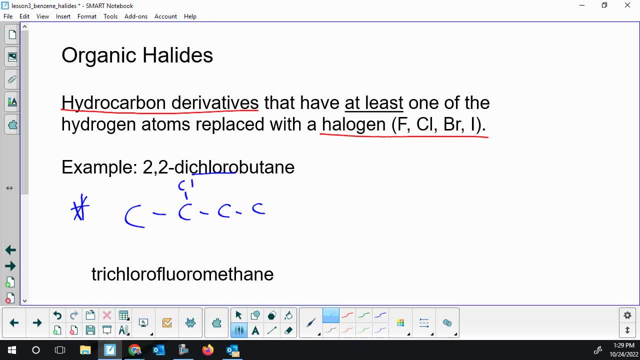 Then I have to go to the second one and put another Cl. I could go up, but I've got more room so I'm going to go down with the second one. That's it. I fill the rest of the bonds in with hydrogen. 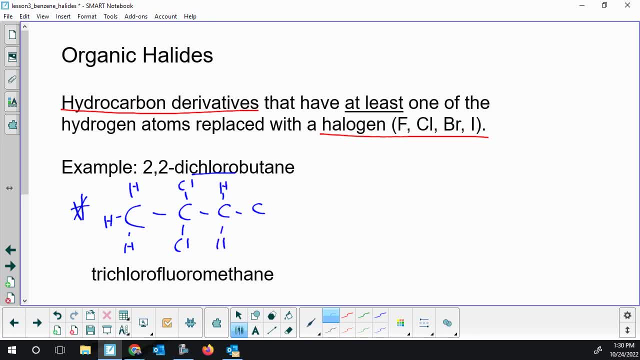 This hydrocarbon derivative has a fair bit of hydrogen left. It is saturated, It is filled up. There's no double or triple bonds here. It's a derivative. There's no benzene here, so this is not an aromatic compound, It's not even a hydrocarbon. 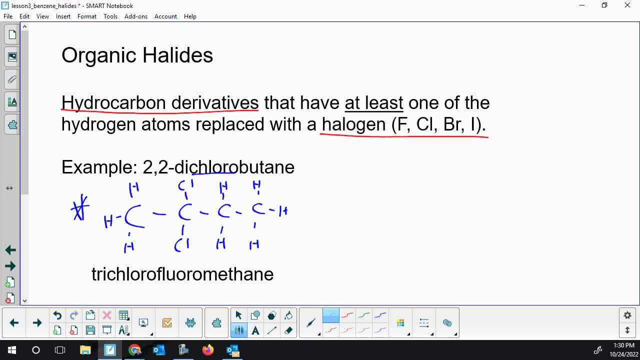 Line structures have a few nuances. Let's do a line Same, beginning: Four carbons, One, two, three, four. lift Again the zigging and zagging is coming from VSEPR theory. None of the bond angles are straight, so you're not. 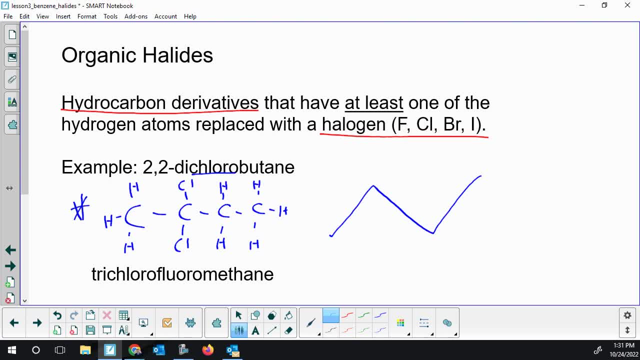 seeing a straight line C's and H's. we never wrote in. We never wrote a single letter yet. but when you have something other than C and H, you have to explicitly write it. On the second carbon, we have two chlorines. That is going to be our second. 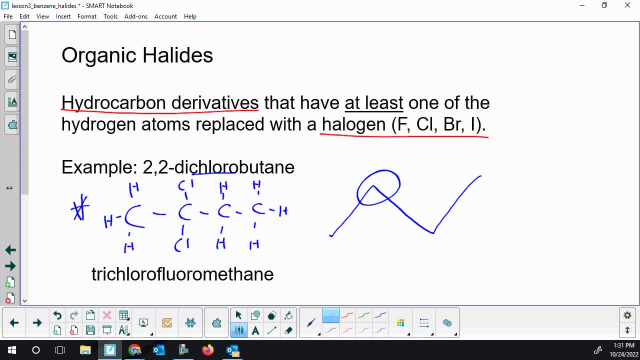 carbon. I want to take that circle out. Second, from the left, I have to put in two chlorine atoms. There's one chlorine and that's the most common way. You'll see it on a test or in a book. Again, you could have went one up and 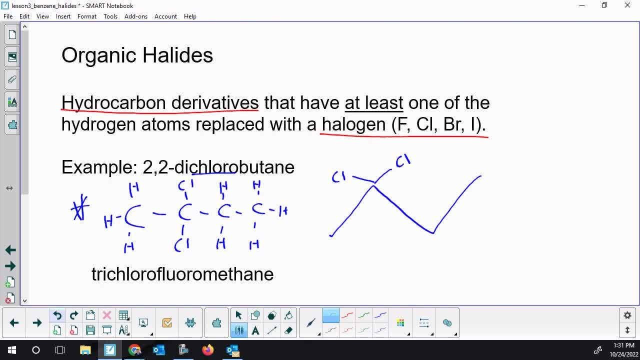 one down. It's not flat like this in real life. This is a flat projection of something that is really tetrahedral. That's why, as long as you have the right connections, it doesn't matter, because we can't draw three-dimensional structures on our 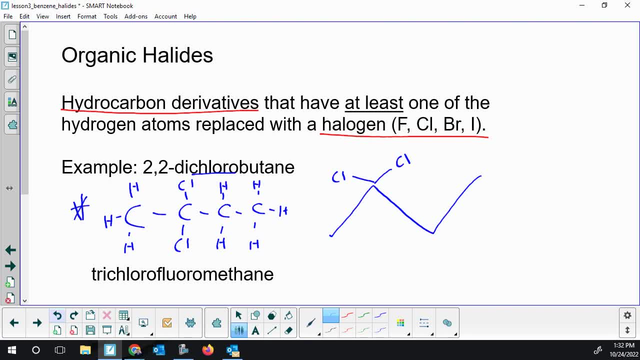 two-dimensional paper. That would be the line, How the line structures work. if you have the end of a line segment and there's nothing there, it's a carbon. If at the end of a line segment you have an atomic symbol, there's. 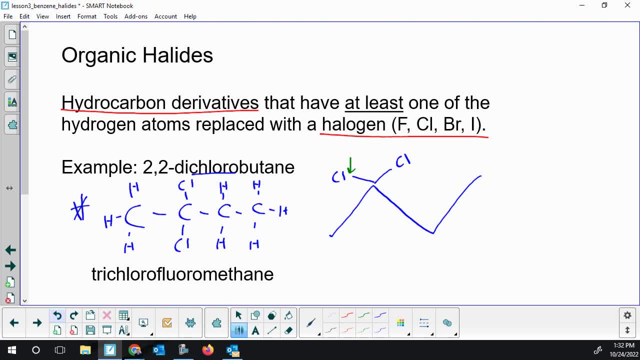 no carbon. at the end of that line segment There is just whatever atom matches that symbol. At the end of that green arrow, there's no carbon there. It's a chlorine As we work our way through organic halides and alcohols and carboxylic acids. 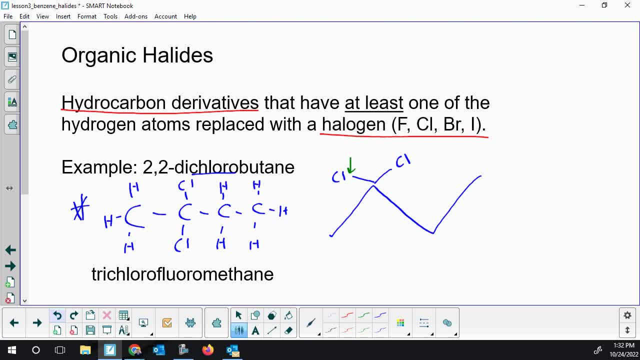 and eventually esters. we're going to be writing in chlorine, bromine, fluorine, iodine and then oxygen atoms. Last I'll do the condensed structure and then I'll do that bottom example. At the very end we have C with three H's. 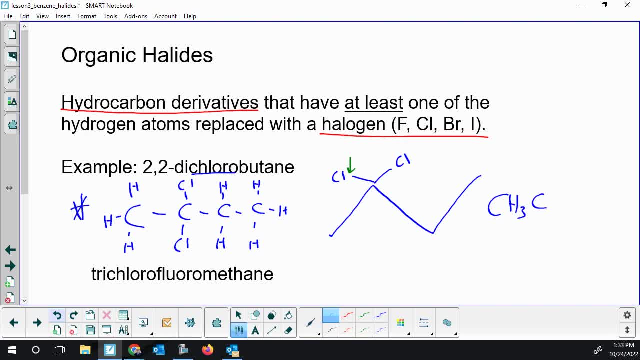 Then we have a carbon. We're going to keep doing the same thing. we just might have to do a C count, sorry, a hydrogen count and something else. There's no hydrogen there, so we only have to do a chlorine count. 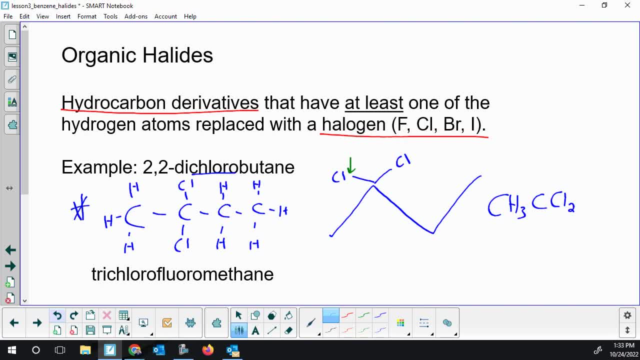 Carbon with three H's, a carbon with two Cl's and then a carbon with two H's and then a carbon with three H's. That's a fully condensed structure. Now we've got something with no numbers. We've dealt with this before It means. 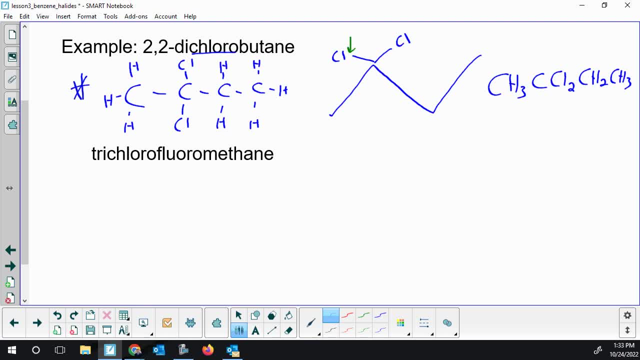 the number was redundant. There's only one possibility, so we're not going to write it: Trichlorophyll fluoromathane C comes before H, so that's why the chlorines came first and the fluorines came second. 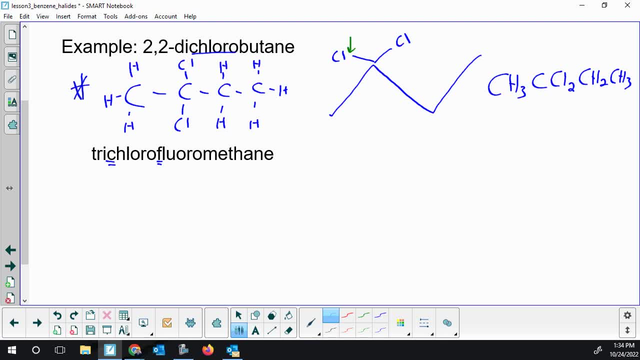 Trichlorofluoro, so Cl and F. We don't start there. We start with the stem or the parent, which is meth, Methane. of course there's actually no single bonds, but we keep the ending ane, even with meth. 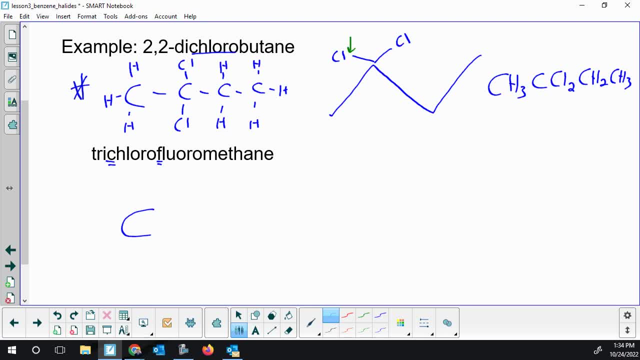 There's no carbon-carbon bonds at all. We don't need numbers, because there's only one carbon. Of course they're all ones. You couldn't have any number but one. All of those four atoms have to come off our carbon, Where you put them, doesn't? 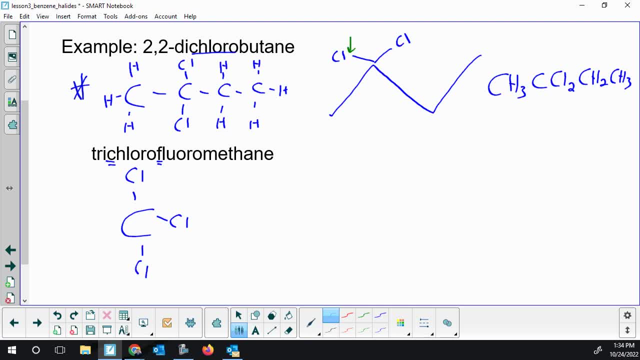 matter. There's one chloro, two chloro, three chloro, there's the trichloro and there's the fluoro, or any rotation of atoms. That would be trichlorofluoromethane, Condensed structure.